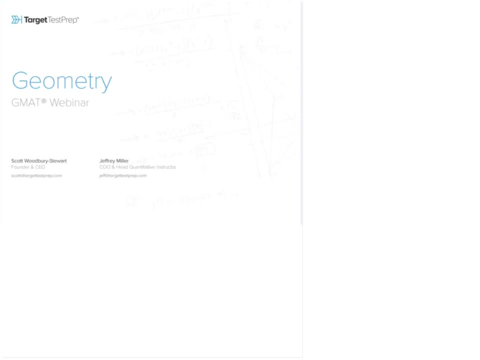 bit about how angles and sides interact within a given triangle, And we can draw a few different triangles out. One of the first ones that we can simply start with would be one that people are pretty familiar with, like the isosceles triangle. Now, the isosceles. 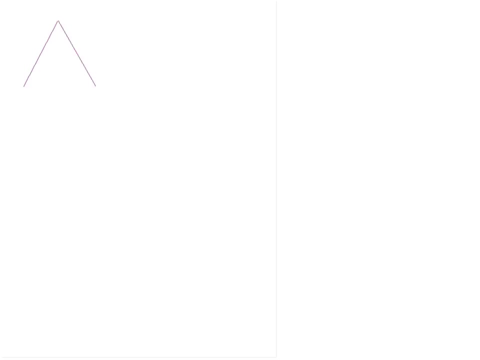 triangle- and keep in mind, none of my drawings are going to be the scale- is a triangle that has two equal sides. So if we're calling this isosceles triangle ABC and we want to make these two sides the same, well, what that means is that angle A here and angle C here. 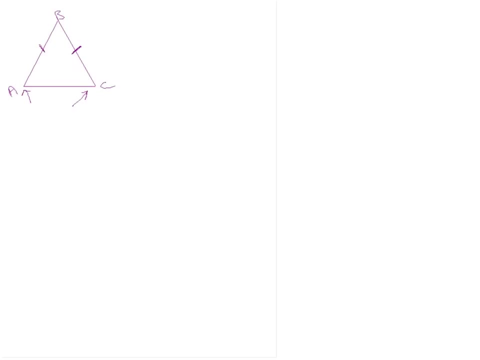 have to be the same angle. So, for instance, we can make them any degree measurement we want. We could say this is 50 degrees and this is 50 degrees, and then that would leave a grand total of 80 degrees for angle B. 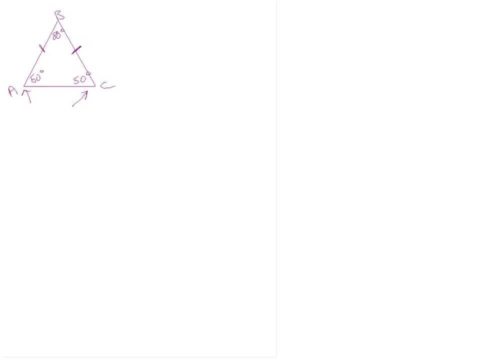 Now what's interesting is you have two equal angles of 50 and 50, and you can see their corresponding sides are equal. What's also interesting- that goes beyond this, but it's kind of in the same light- is that the largest angle in a given triangle is always opposite. 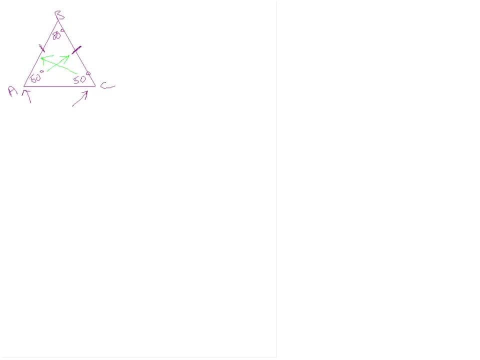 the largest side. The smallest side is opposite the smallest angle. So an example of that- and we're going to kind of get into this in a second- is, let's say we have a triangle like this, And obviously this is a triangle we don't see too much of, but you can see. 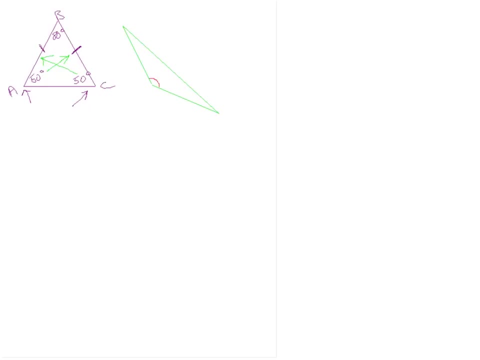 this angle here is clearly the biggest angle in the triangle. We'll call this angle C, And you'll notice that angle C is the largest angle in the triangle, And so that's sort corresponds with what we could easily see as the largest side. 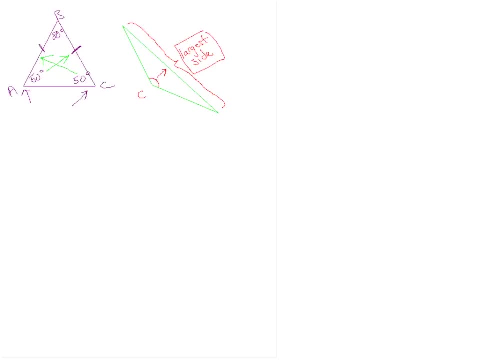 Now the GMAT expects you to know this, Thus they will test you on it. So the first thing I want to do tonight is I want to give a question- that's testing- on that idea, and then we're going to continue forward. 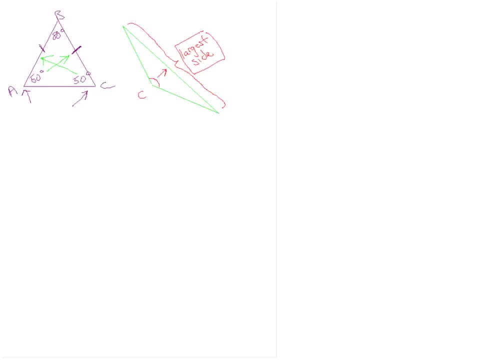 and do some stuff on different problems where simplifying triangles is tested. So let me get the first problem up And then we can go from there. Okay, for the sake of this problem, we're just going to have the Roman numerals up. 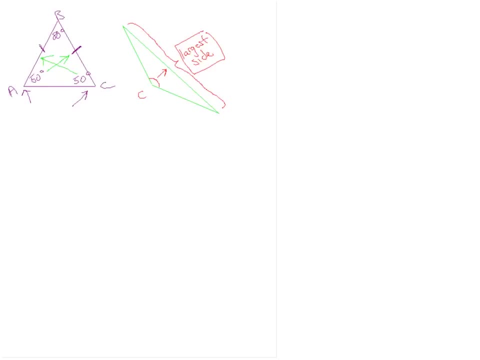 And I'm posting it right now. Okay, so, like always everyone, I'm going to give you about two minutes And keep in mind, you know, any of these Roman numerals can be answer choices, and then we will go from there and talk about it. 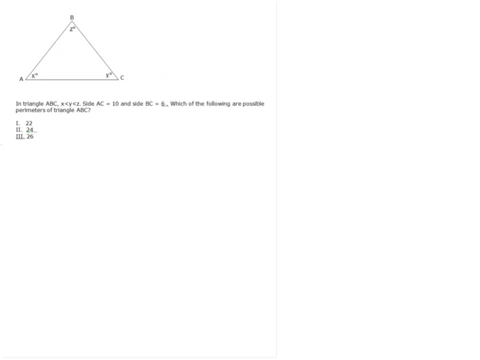 So I'll give everyone two minutes And as you get your answer, as always, you can put your answer in the public chat so everyone can see you know what different people are getting. Okay, Okay, No problem, I'll move up a slide. 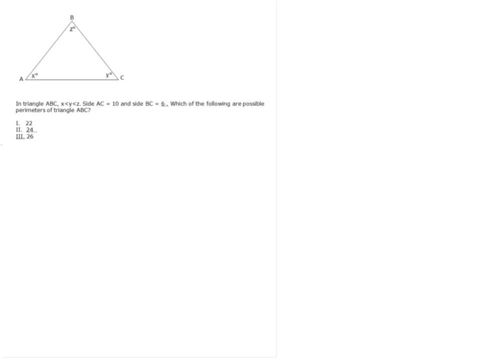 Okay, Okay, All right. So I'm always excited, and I'm excited to answer your questions, Because I know a lot of times when I'm thinking of things, I forget to do it, But I think that's what's so important about this project. 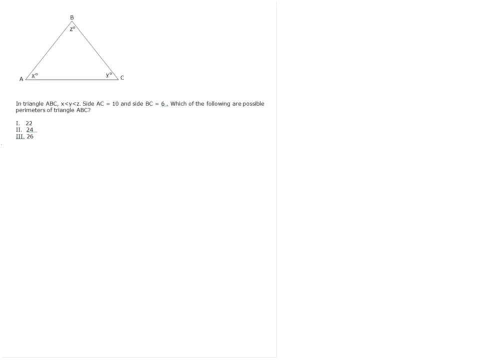 is that you know the many things that we talked about. we're going to put the answer in the public chat and, by the way, we're going to do it in a very simple you, you, okay. so that was about two minutes and you know one of the things i bring up a lot and and i know, 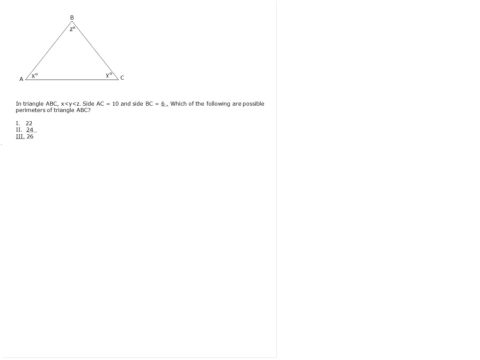 scott does too, is that a lot of times in gmap problems. uh, regardless of topic, really, you're going to always see small pieces of information and sometimes it's easy to ignore that information. you know, for instance, in a problem like this, where it says in triangle abc, x is less than y, which is less than z, it's possible that. you know you. 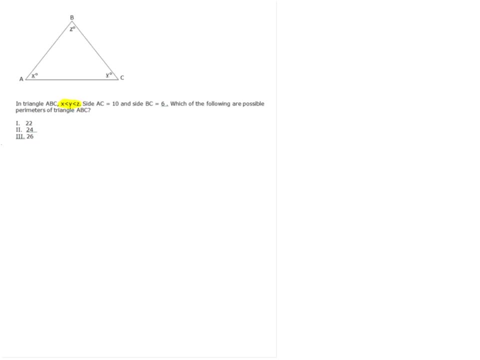 could look at that and completely glance over it, but the problem is is that that's actually a really critical component of this problem, and if you don't actually read that and internalize it, you may not know where to go from here. so what's so important about this is that this is actually giving us the relative 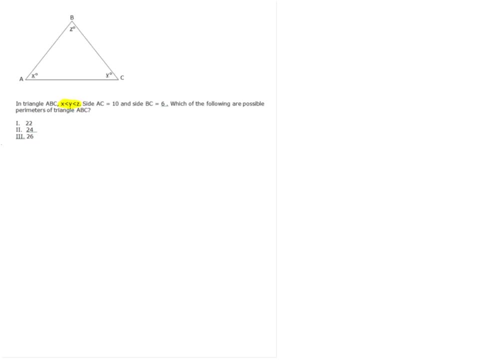 size of each individual angle. so what we know is that x is actually the smallest angle, so i'll put a little s next to it. y is- we'll call it the middle angle as far as size is concerned, so i'll put an m and z is the largest angle now, as, as everyone recalls from what i just said. 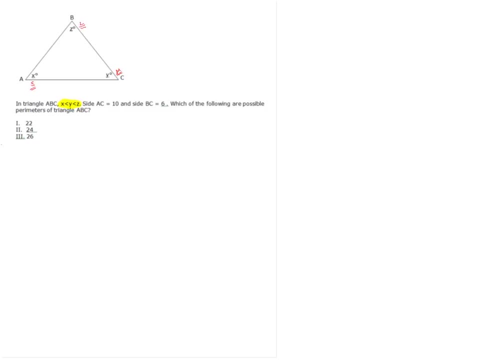 angles and opposite sides correspond. so that would mean that side ac is going to be the largest side. so we'll write it up here. that means that side bc, which is opposite angle x or the small angle, is going to be the smallest side. so what is the mid-range side? well, that's obviously. 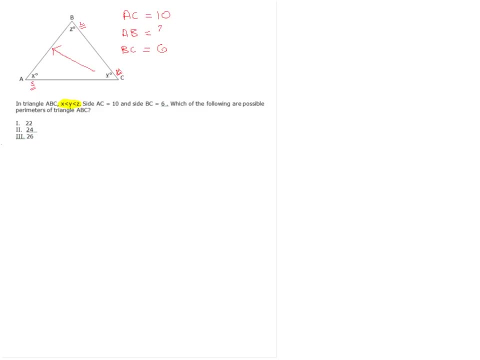 a, b, and that's obviously what we're being asked about. so now, if we look at the table, we're going to get the 대방산, 산하 австри단. that's the big picture of what the matrix is. then we're going to get the mid-range side. 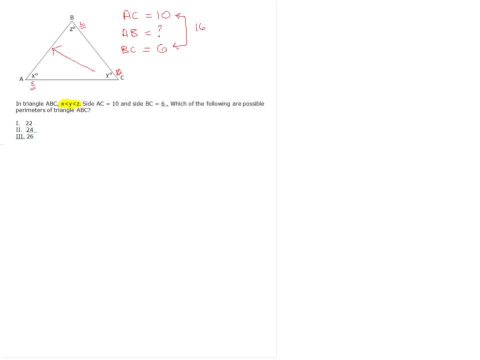 the one side of that is a, b and that side is going to be the farthest side and the other side is going to be that side a. and let me show you how this works. my tutorial is not actually telling you what side side i've just given you the real deal is because we're not seeing a, c and that's the. 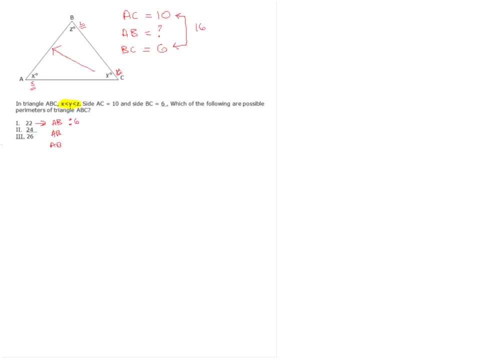 real issue. it's not saying which side side is going to be the farthest side. and then we're not seeing. If the perimeter is 24,, that makes AB 8. And if the perimeter is 26,, that makes AB 10.. Now, according to what I taught everyone, 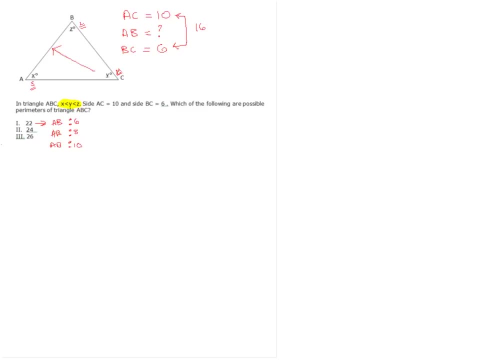 AB must be between 6 and 10.. So right away you can see that you can get rid of the 6, and you can get rid of the 10.. So the only possible option here is Roman numeral 2 for the side of AB. 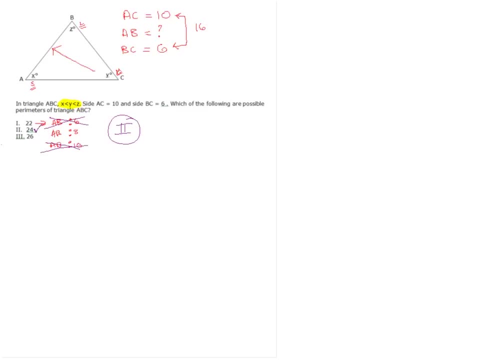 Or in other words, the only possible perimeter here is 24.. So this is kind of a good warm-up question that's getting everyone into the idea that in triangles, sides and angles have a lot to do with each other. So we have to be very careful there. 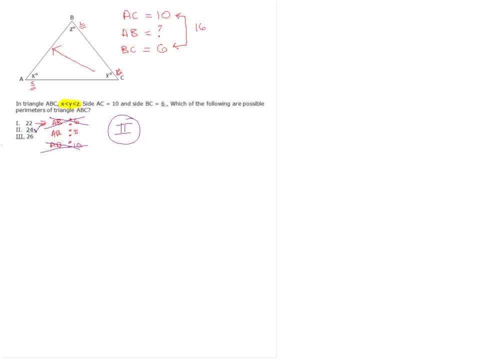 Now I'm going to kind of step it up a level for the next question, Because in the next question we're going to learn a lot about not only how sides and angles correspond, but also, or furthermore, how the GMAT will give you. 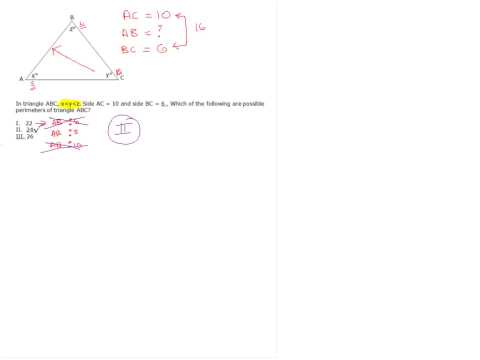 a few angles and triangles and expect you to simplify them prior to answering a question. So what I want to do here is get this posted And I will give everyone again two minutes to get through this And keep in mind everyone. this is data sufficiency. 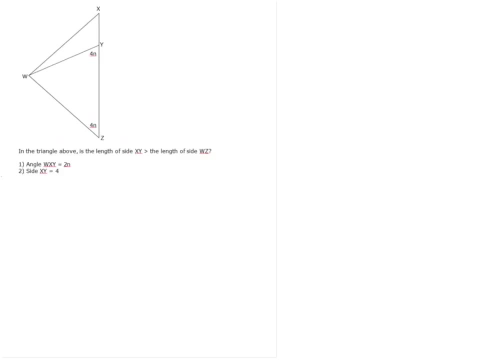 But as always, we don't have the answer choice listed And you may have to scroll down just a touch Just to see the two statements. So you may have to scroll down And if you have a question that you don't get, 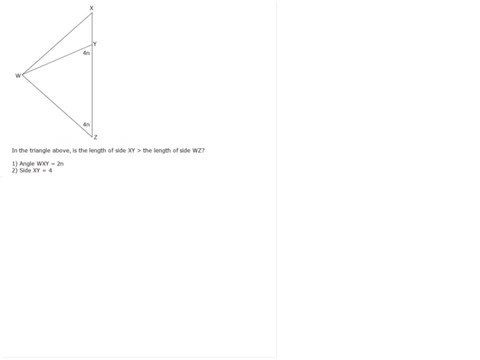 then you have to go to the data sufficiency tab And we'll put the link in the description below And then you can go ahead and click the next question, And that way we can get to the next question. You can also go ahead and click the next question. 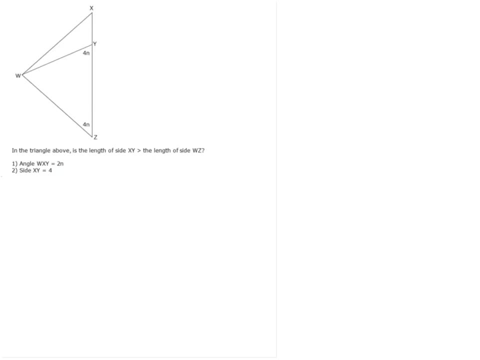 And you can see that we have a couple of options here. So we're going to go ahead and click the next question, And then we're going to go ahead and click the next question. you, you, you okay. so that was a little bit over two minutes actually, but this is a 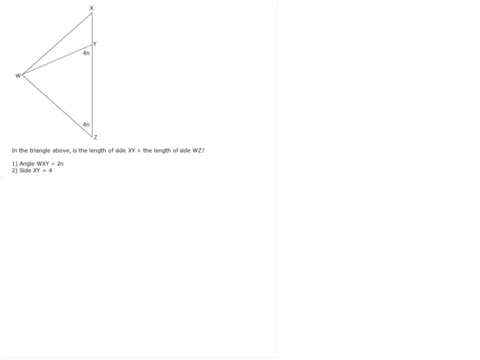 um, this is a pretty intense question so i wanted to give everyone enough time to to to to try it out, and you know this is one of my favorite geometry questions. um, you know that we have, and i really like it because it's testing- a lot of things that i feel are common and high. 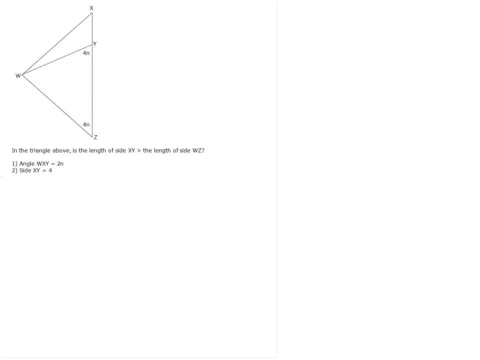 level triangle questions um on the gmat. and the reason i say that is because the only way you're going to be successful on a problem like this is if you immediately start simplifying. you know, if you take this diagram and you just leave it as is, then you know you, you're probably not going to get too far in this. 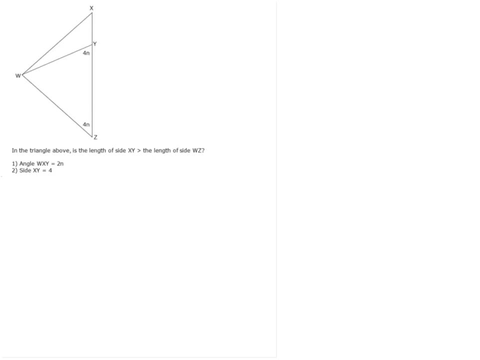 question and in fact this is going to be a very annoying question for you. but if you can kind of have that keen eye in geometry, especially in triangles, to see when the gmat has left the door open for you to put in some extra work, life is going to get a lot better, even on on what i. 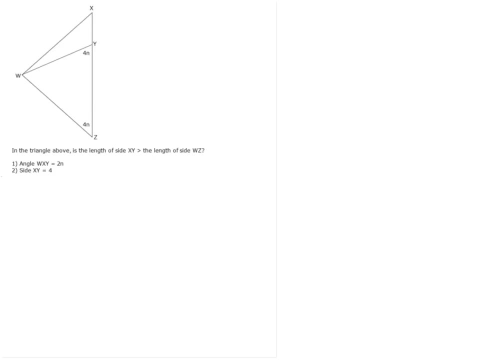 consider high level questions like this. so you know, immediately upon seeing this question, the first thing that my eyes lay it lay on is the fact that i have a four end angle here and a four end angle here. now, based on what i just discussed, that means we're dealing with an isosceles triangle. so 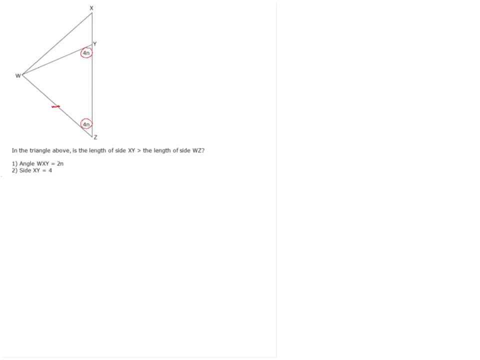 we can kind of denote that yz or, excuse me, wy- is equal to yz. now there's more than just that. the other thing is that we can start simplifying angles. now, remember, there is a grand total of angles, like of 180 degrees in any triangle. so if we look at triangle W Y Z, let's say we want. 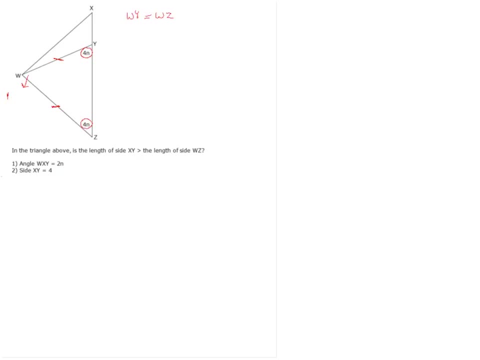 to simplify what I'll call angle W. well, that's simply 180, which is the total degree measurement of a triangle, minus the sum of the other two angles, which is 8n. and then we can't forget about this angle here, which we can call X, Y, W. 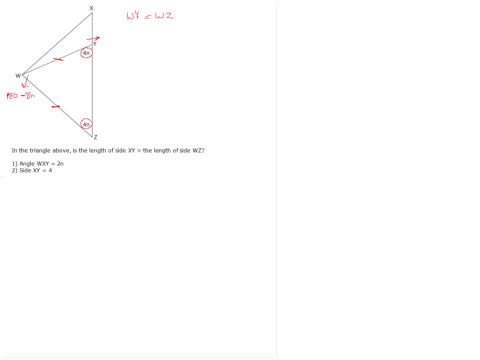 because it's on the same plane with the 4n. we know any straight line has a total degree measurement of 180, and thus we get to say that this is 180 minus 4n. now, to be clear, this is the stuff you want to be looking for in a question where 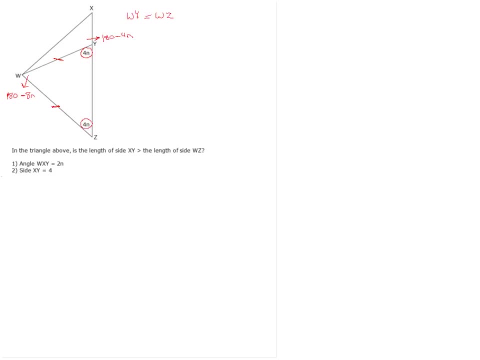 they're providing angles and they're leaving space open for you to simplify. of course, the question that we're dealing with is: is side X, Y greater than side Y, W, Z? so we want to keep that in mind. now, what statement one tells us? and it just: 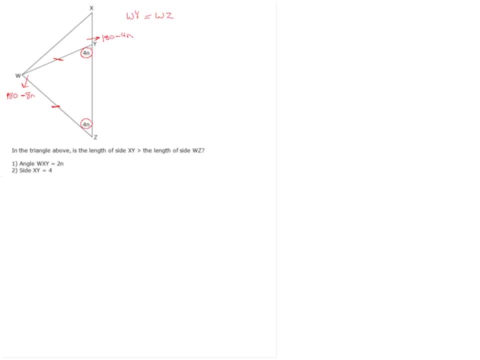 scroll down a little bit, you'll see it is that angle W, X, Y- and I'll just write it at the top- equals 2n. now again, we want to first plug that in, and you know. one other thing to mention is if you are on an actual GMAT. now, obviously I have the. 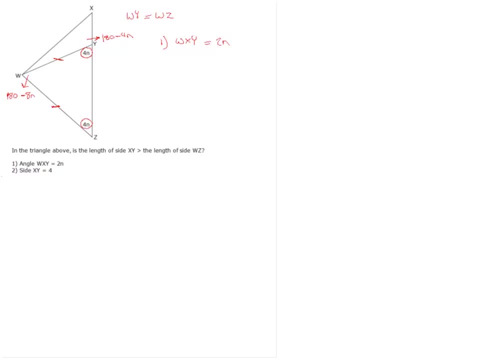 screen. here I can write next to my shape. this is definitely something that you're going to want to sketch out, so you're never going to want to just look at the information on your computer screen and then extract it on your page, but rather you're going to want to write out this entire diagram for sure, okay, so 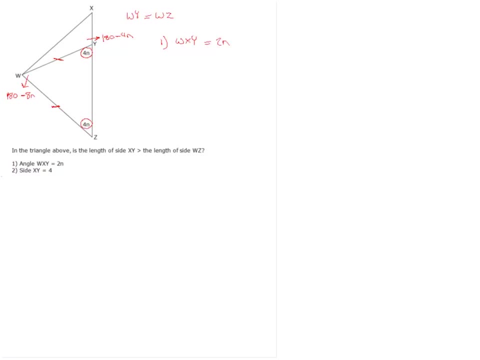 we see that W, X, Y is 2n. now what that means for us is that we have two out of the three angles of our triangle here, so we and do the same thing we did with the larger angle, W, is we're going to do with a? 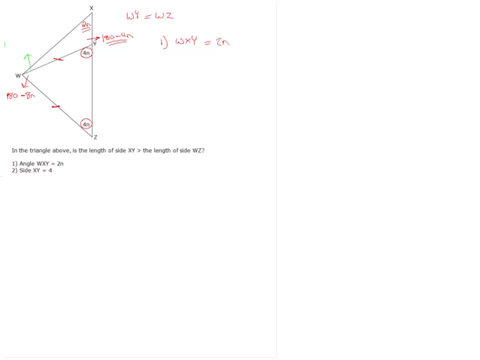 smaller version. so what we're going to say is that that's equivalent to- and i'm doing this in green- 180 minus the combined sum. and this is where you have to be really careful, and this is why i put these brackets in, because i see students make this mistake all the time. add this together first, and 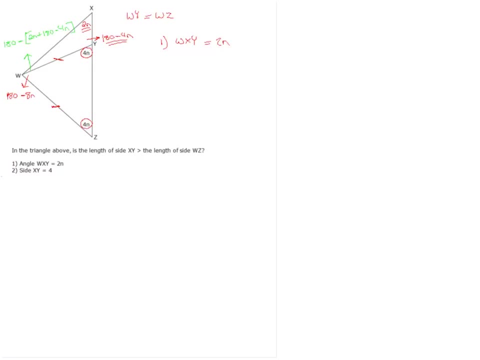 then subtract it, because without those brackets, just so you can see it, you have no idea really what you're subtracting. but with the brackets you know that first you're adding all this stuff together. so this gives you 180 minus in brackets, negative 2n plus 180. i'm running a little bit out. 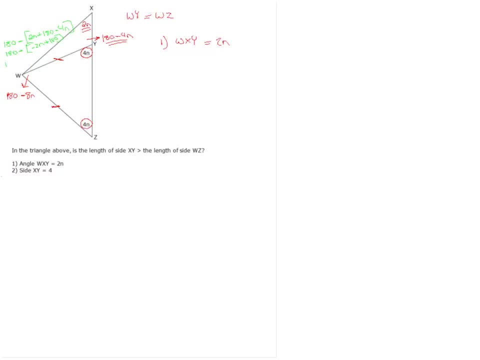 of room. so i'm just going to take my arrow off and this becomes 180 minus. and remember, now you're distributing the minus sign within the bracket. so actually that makes it a plus 2n, minus a 180, and after all that work we're left with 2n here. now this is: 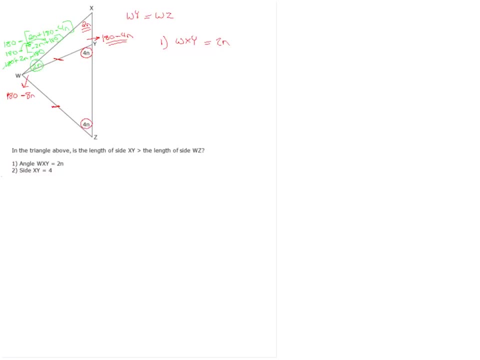 extremely important because we have a 2n there which i'll highlight, and we have a 2n here. so what triangle wxy is? and keep in mind this probably should have been said that it wasn't drawn to scale because clearly it's not um that we have an isosceles triangle. 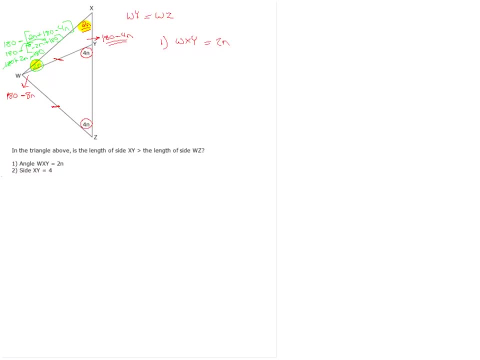 and so what we do is we go opposite that angle, which i'll do in a different color- and we see that side x- y is also equivalent to side y- z. now, if x- y is equivalent to y z, then it also- excuse me- to w y, then it also has to be equivalent to y z. so here's what we know. we know w y. 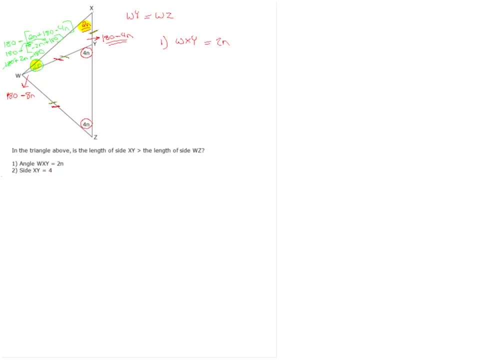 equals y z, which equals x y. and this is super, super important because if we go down to the question, it says: because we know w y is equal to y z and because we know that means w y is equal to y z, and we know that x and y are the other vanes of the equation. so that's going to be wild, so we're only going 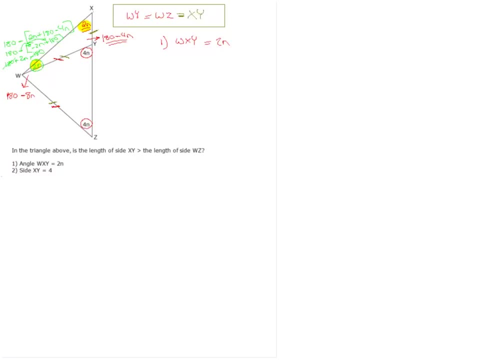 to be going through the question, so we're going to go through the next part of the question. so we've got some. It says: is the length of XY greater than the length of side WZ? Well, clearly we can say the answer to that is no, because they're equal. 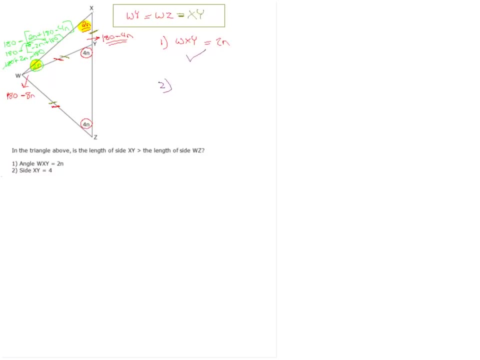 So that makes statement one sufficient. Now, statement two, on its own, is simply telling us that XY is four, without having any other information because, remember, we know nothing about these angles. That's simply giving us one of the sides here, and that's definitely not enough information. 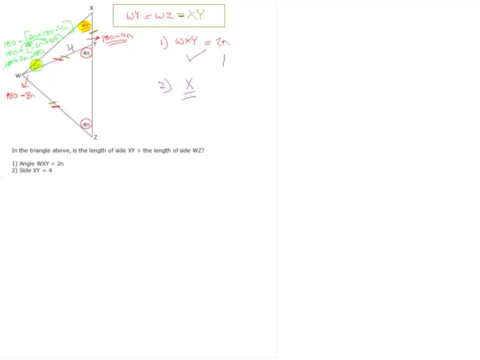 So this leaves us with statement two being insufficient and the answer here being A. So if some of you struggled with that and you thought this was a lot of steps, keep in mind this is a high-level question, You know, when you see something like this, 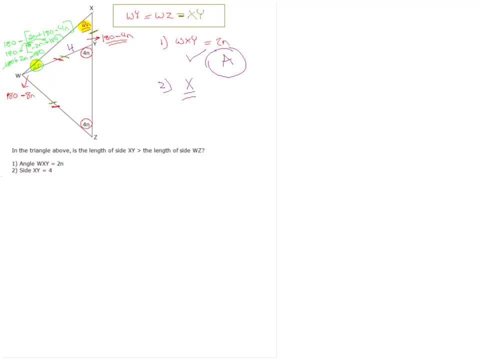 GMAT is definitely expecting, you know, a very high level of detail from you to be able to get through this question. So the last thing I want to cover tonight is I want to talk about the question of how to get through this question. 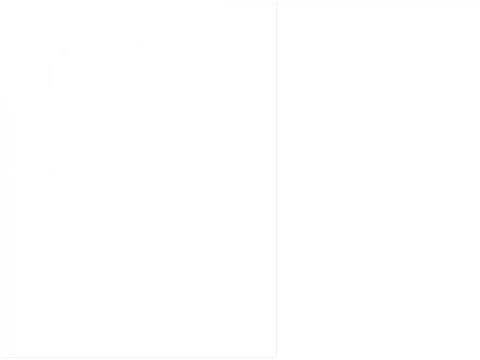 So there are two different types of right triangles that you're expected to know in the GMAT, You know? the good news is you don't have to know any trigonometry on this test, which is nice, but a few things that stem from trig. 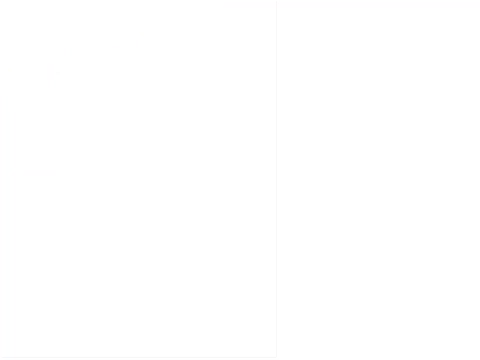 are some of the right triangles that they expect you to know and some of the side angle relationships that you're expected to know. So two popular ones- and I'm sure most of you know exactly what I'm getting at- is the 45-45-90 and the 30-60. 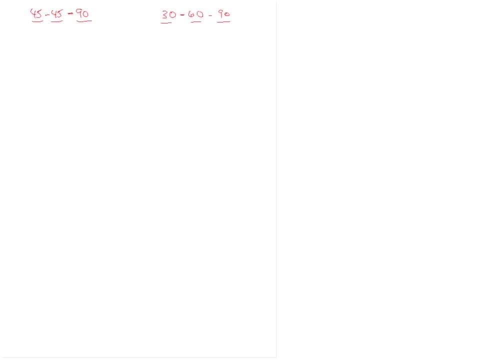 The beauty of this is that once you know either any two angles or any two sides, you can tell right away if you're dealing with a 45-45-90 or a 30-60-90.. Now remember my triangles. I'm just drawing them out. 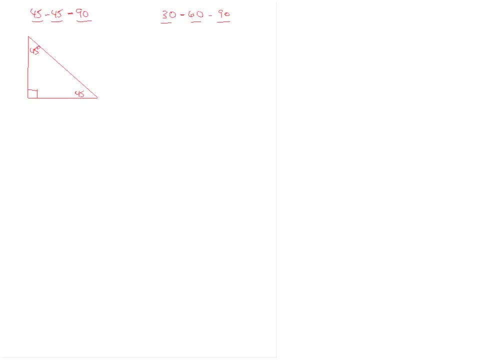 I'm not trying to make them to scale The 45-45-90,. what we need to know is that if we're talking about the side ratios, the side opposite the 45 is X. the side opposite the 45 is X. 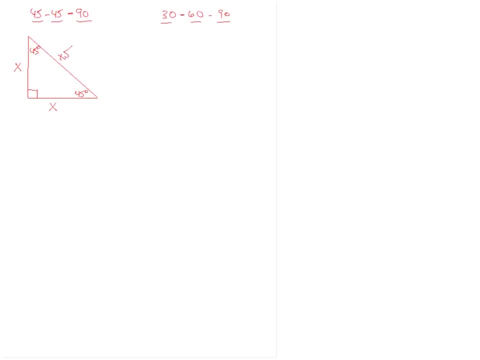 and the hypotenuse or the side opposite, the 90, is X-root-2.. For the 30-60-90, the ratios are slightly different. We've got the 90-degree angle here, 30-degree angle here, 60 here. 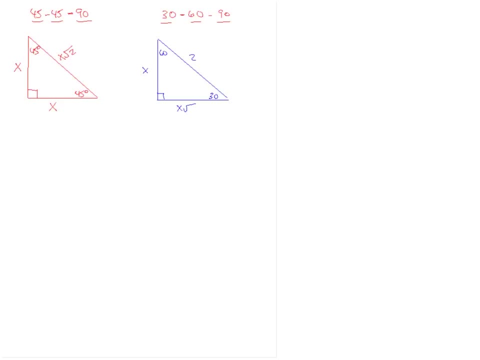 We have X, X-root-3. And then 2X. So what we're going to do is we're going to do a couple problems that are tested on this, and then we're going to go from there and I'll be turning this over to Scott. 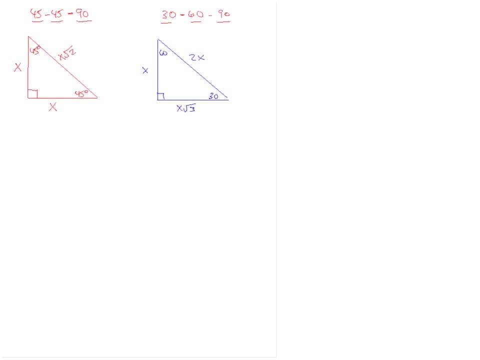 Okay, so I'll give everyone two minutes here, All right, Okay, so we do have s-d傷, so we get 1 feet here, Divi. So this is 1, 0,. this is 1, 0, 3, 3, 4, 1, 5, 6, 7, 6, 7, 8, 9, 10, 11, 10, 11,, 12,, 13,, 14,, 14,, 15,, 16,, 17,, 18,, 19,, 20,, 21,, 22,, 23,, 24,, 25,, 26,, 27,, 28,, 29,, 30,, 31,, 32,, 33,, 32,, 34,, 34,, 35,, 36,, 36, 36,, 37,, 39,, 40,, 40,, 41,, 42.. 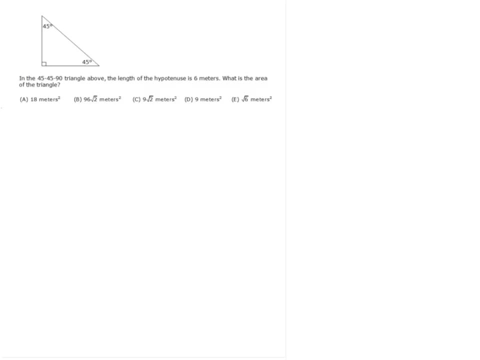 And again, we got an elsewhere when we broke that Мы да Petra, and we had an elsewhere when we broke that Мы да Popありがとうございました, And we got back at our schedule. So, 2016, that was a 4182, and then, while we're doing this, 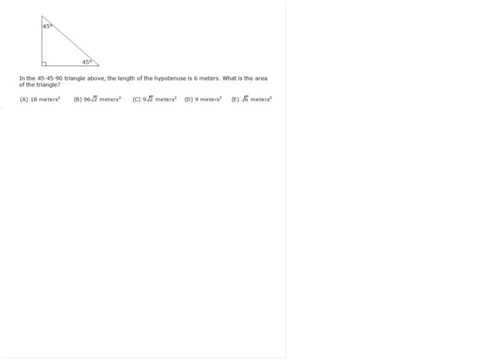 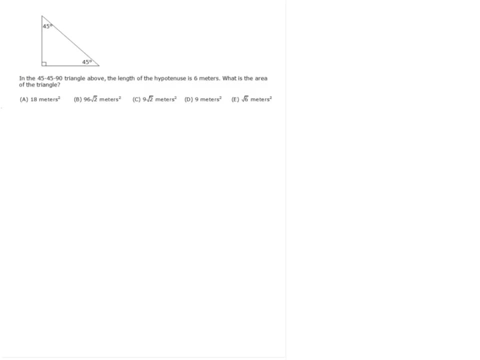 a little bit over two minutes, but this one you know if you are following one. you know if you are following one. you know if you are following um the rules i just taught it shouldn't um the rules i just taught. it shouldn't um the rules i just taught. it shouldn't be too bad now. 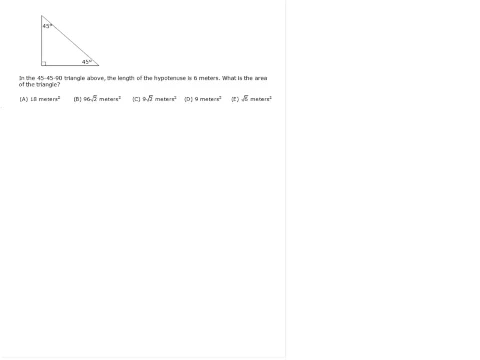 be too bad now. be too bad now. one of the things i never mentioned, one of the things i never mentioned, one of the things i never mentioned about the 45 45 90 triangle, about the 45 45 90 triangle, about the 45 45 90 triangle one. it's actually the same thing as 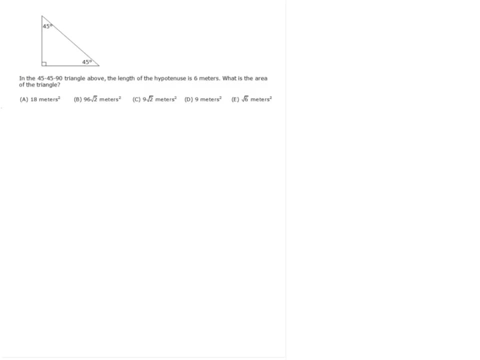 one, it's actually the same thing as one. it's actually the same thing as half of a square. so if i were to just half of a square, so if i were to just half of a square, so if i were to just add a square here, add a square here. 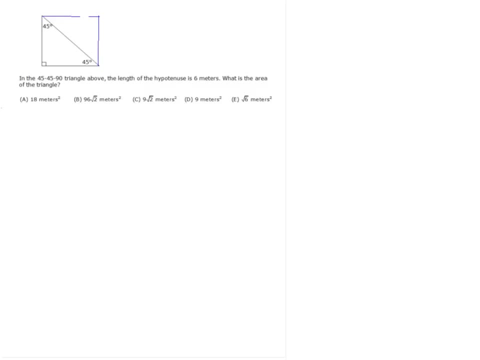 add a square here. there you go that half of a square. so there you go that half of a square. so there you go, that half of a square. so these rules apply to when you hear the. these rules apply to when you hear the. these rules apply to when you hear the words diagonal of a square, which 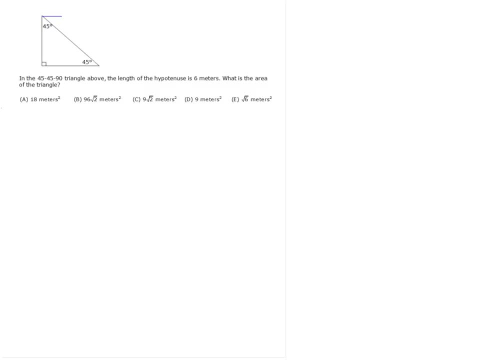 words diagonal of a square, which words diagonal of a square, which is also tested. the other thing is with is also tested. the other thing is with is also tested. the other thing is with this type of triangle. if you truly this type of triangle, if you truly this type of triangle, if you truly needed to, you could use the pythagorean. 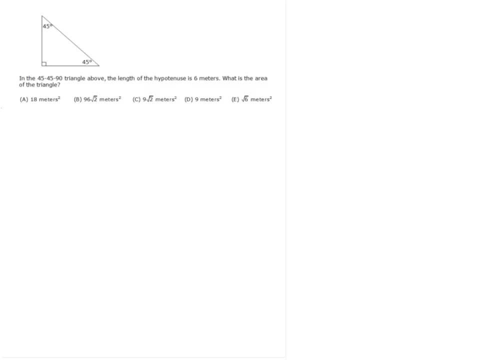 needed to, you could use the pythagorean. needed to, you could use the pythagorean theorem, but theorem but theorem. but obviously if there's a shortcut to do, obviously if there's a shortcut to do, obviously if there's a shortcut to do something on a timed exam. 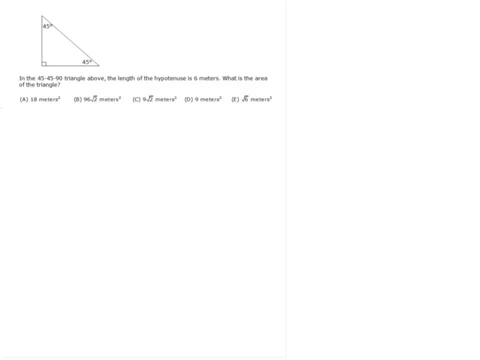 something on a timed exam. something on a timed exam? it's a no-brainer. use the shortcut i. it's a no-brainer. use the shortcut i. it's a no-brainer. use the shortcut. i realize that this on top of every other. realize that this on top of every other. 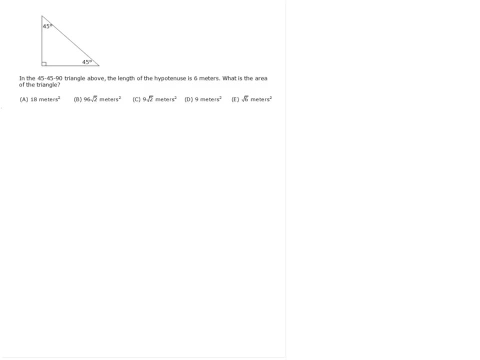 realize that this, on top of every other thing that you're told to memorize, thing that you're told to memorize, thing that you're told to memorize- can get overwhelming, but you know that's can get overwhelming. but you know that's can get overwhelming, but you know that's why the flash card was created and i why the flash card was created and i why the flash card was created and i know as long as you have it there, and know as long as you have it there, and know as long as you have it there and you're able to review it from time to. 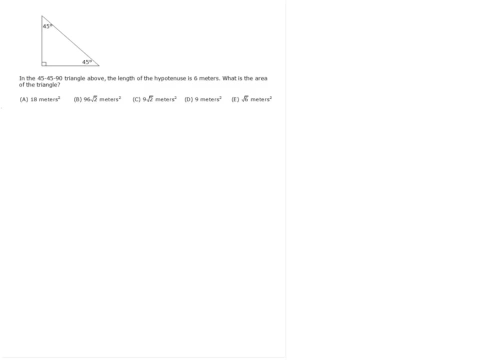 you're able to review it from time to. you're able to review it from time to time, time, time. this is something you probably will not. this is something you probably will not. this is something you probably will not forget. so, if we're going back to forget, so, if we're going back to 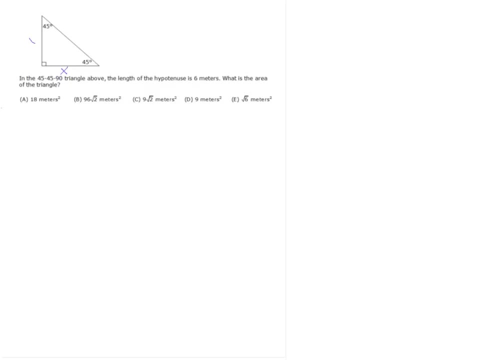 forget. so if we're going back to our side angle ratios, here we have x, our side angle ratios, here we have x. our side angle ratios. here we have x, we have x, we have x root, 2. the first: we have x, we have x root, 2. the first. we have x, we have x root 2.. the first thing you're going to do is you're thing you're going to do is you're thing you're going to do is you're going to do anything possible to solve, going to do anything possible to solve. 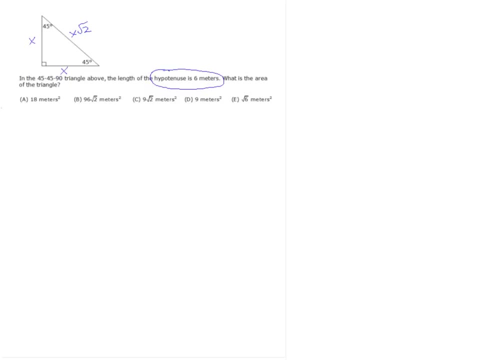 going to do anything possible to solve for x, for x, for x. notice: here the hypotenuse is six meters. notice: here the hypotenuse is six meters. notice: here the hypotenuse is six meters. so you say that x root 2, so you say that x root 2. 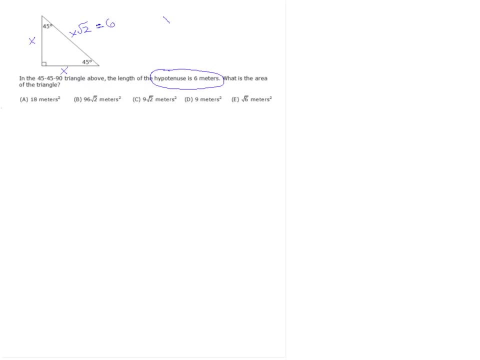 so you say that x root 2 equals six. what's the purpose of that equals six? what's the purpose of that equals six? what's the purpose of that? well, now, with that equation which i'll well, now, with that equation which i'll. well, now, with that equation which i'll write. 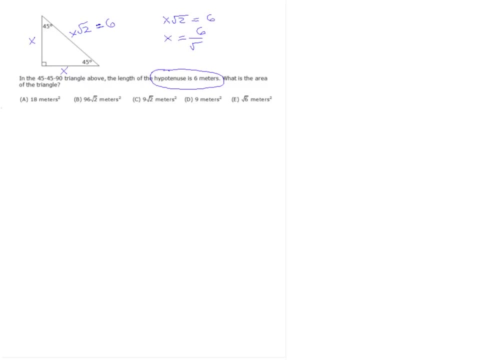 write, write on the side. we can see that on the side. we can see that on the side. we can see that we have a value for x now. we have a value for x now. we have a value for x now. the next thing i'm going to do is not. 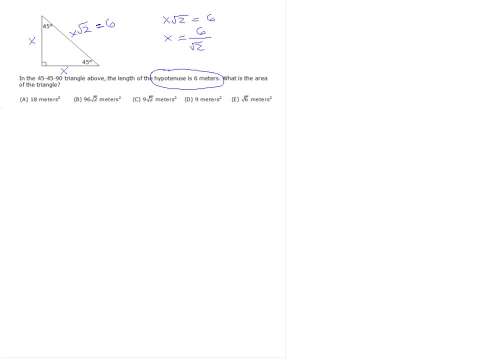 the next thing i'm going to do is not. the next thing i'm going to do is not mandatory, but it's something that's mandatory. but it's something that's mandatory, but it's something that's probably going to help you, probably going to help you. 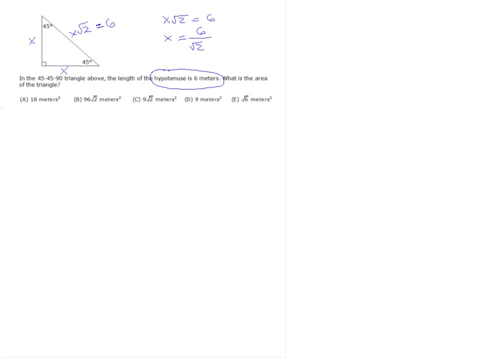 probably going to help you. because nine times out of ten your answer. because nine times out of ten your answer, because nine times out of ten your answer: choice is not going to be left. choice is not going to be left. choice is not going to be left with a radical in the denominator. so what? 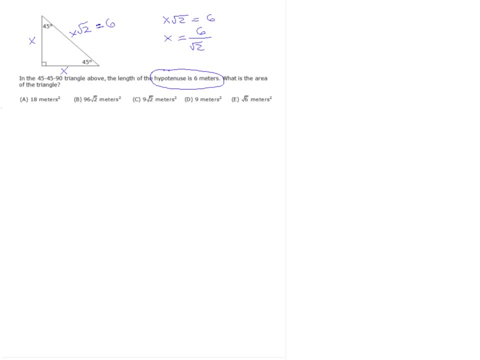 with a radical in the denominator? so what with a radical in the denominator? so what you need to do is you need to. what's you need to do is you need to. what's you need to do is you need to what's called rationalize that denominator. to 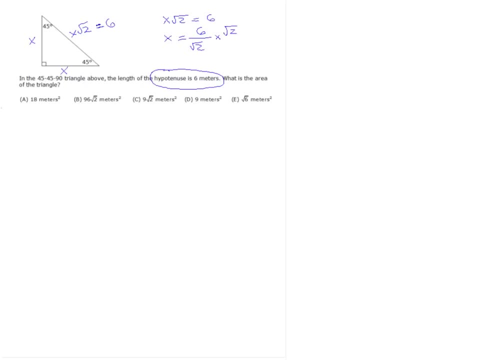 called rationalize that denominator. to called rationalize that denominator. to do that, do that, do that. you're going to multiply by root 2 over. you're going to multiply by root 2 over. you're going to multiply by root 2 over root 2. the reason you're doing root 2. root 2. the reason you're doing root 2, root 2, the reason you're doing root 2 over root 2, over root 2 over root 2 is: first of all, you can't change the is first of all, you can't change the. 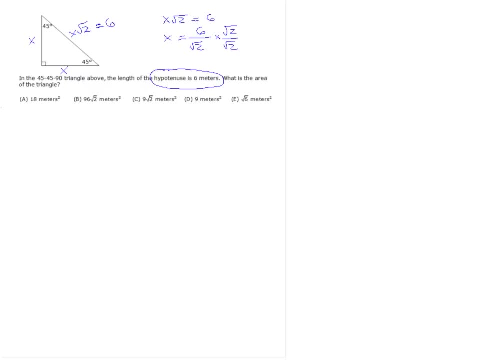 is: first of all, you can't change the value of the expression and root 2 over value of the expression and root 2 over value of the expression and root 2 over root 2 is 1, root 2 is 1, root 2 is 1. and when you multiply root 2 by root 2 on, 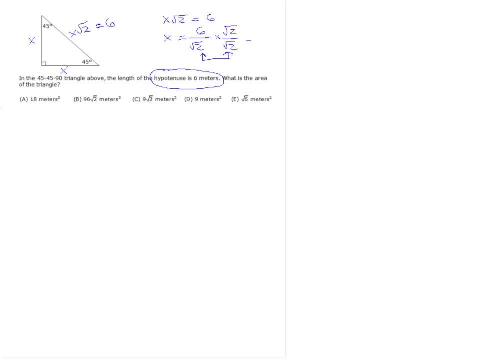 and when you multiply root 2 by root 2 on, and when you multiply root 2 by root 2 on the bottom, the bottom, the bottom, you simply get 2. so now, all of a sudden, you simply get 2. so now, all of a sudden, 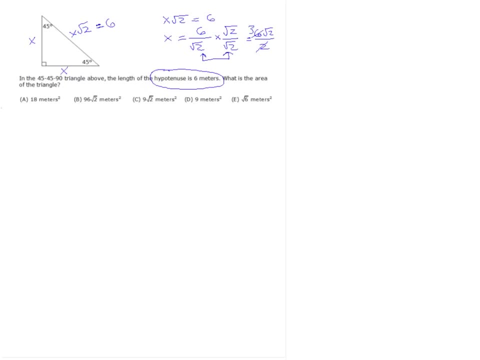 you simply get 2. so now, all of a sudden, your value of x, your value of x, your value of x is this: and if you simplify it down, is this: and if you simplify it down is this: and if you simplify it down, you get x to equal 3 root 2. 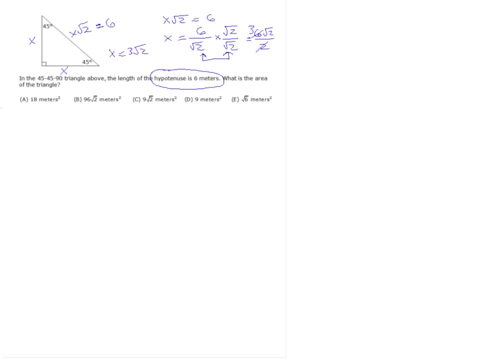 you get x to equal 3 root 2. you get x to equal 3 root 2. so notice, and i'll change the color. so notice and i'll change the color. so notice and i'll change the color here here. here, x is 3 root 2 here. 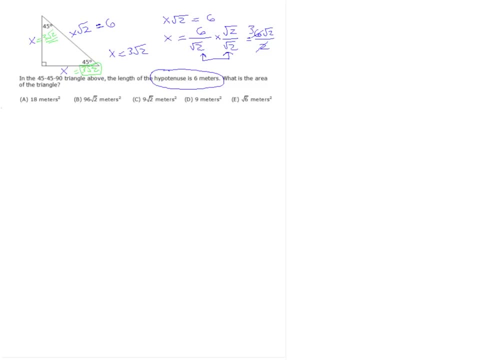 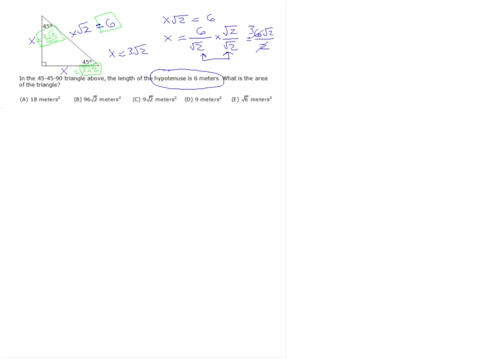 and it's a grand total of six here. so if we are getting here, so if we are getting here, so if we are getting the- oh well, we're only getting the, the. oh well, we're only getting the the. oh well, we're only getting the area of the triangle, good. 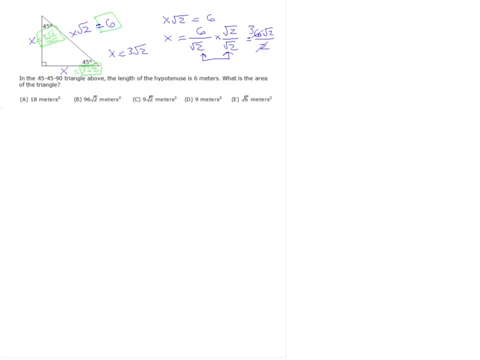 area of the triangle: good. area of the triangle: good, i thought we were getting the perimeter. i thought we were getting the perimeter. i thought we were getting the perimeter, so i just did some extra credit for. so i just did some extra credit for. so i just did some extra credit for everyone. 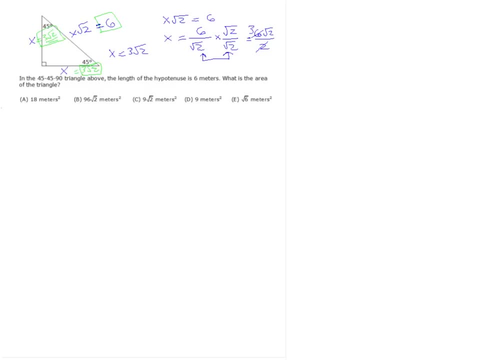 everyone, everyone. so we don't need, we don't really care, so we don't need. we don't really care, so we don't need. we don't really care about six. what we care about is the fact about six. what we care about is the fact about six. what we care about is the fact that 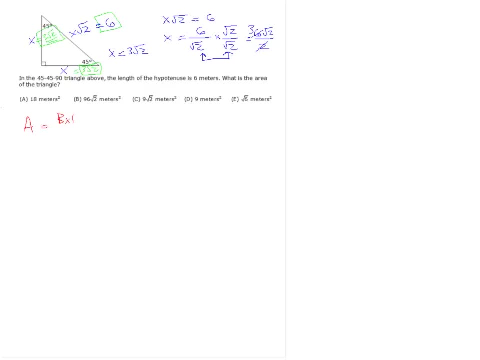 that that area is base times height over two. area is base times height over two. area is base times height over two. now for those who have been reading along, now for those who have been reading along, now for those who have been reading along our curriculum, our curriculum. 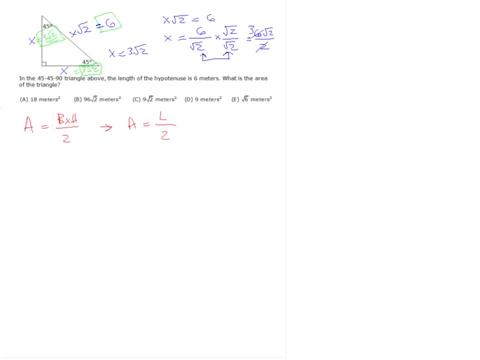 our curriculum. we actually just say l squared over two. we actually just say l squared over two. we actually just say l squared over two. the reason we say l squared, the reason we say l squared, the reason we say l squared, is because our two legs are equal. is because our two legs are equal, is because our two legs are equal, doesn't matter how you do it, you know at. doesn't matter how you do it, you know at. doesn't matter how you do it, you know, at the end of the day it's all going to. the end of the day, it's all going to the end of the day. it's all going to come out of the wall in the wash, come out of the wall in the wash, come out of the wall in the wash, and you should end up with the same. 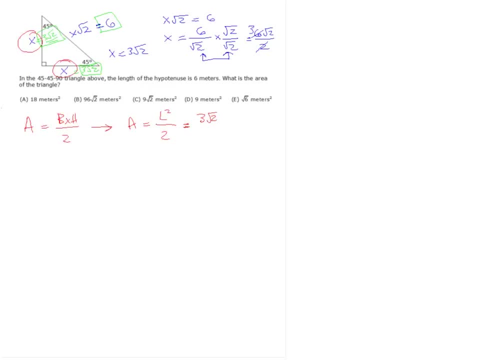 and you should end up with the same. and you should end up with the same answer. so three root two squared over two, so three root two squared over two. so three root two squared over two gives us nine times two, gives us nine times two, gives us nine times two over two, which gives us an answer of nine. 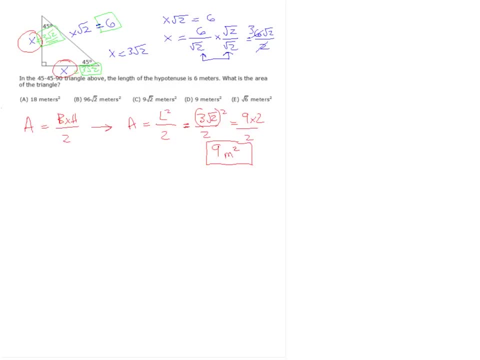 over two, which gives us an answer of nine over two, which gives us an answer of nine. of course it would be meters. of course it would be meters. of course it would be meters, squared so, hopefully squared, so, hopefully squared, so hopefully, for everyone here tonight, what i just 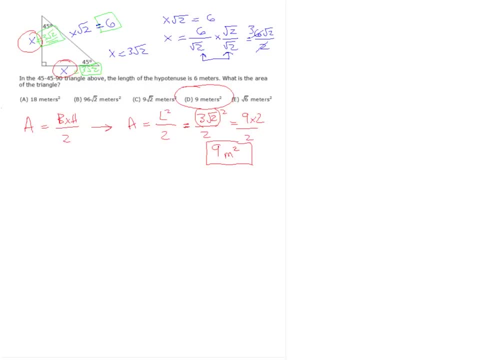 for everyone here tonight, what i just for everyone here tonight, what i just showed you, showed you, showed you, was more or less business as usual, as was more or less business as usual, as was more or less business as usual as far as geometry goes, far as geometry goes. 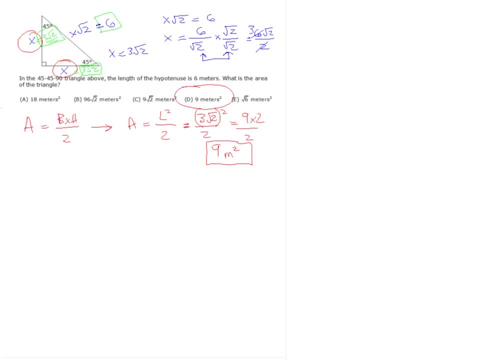 far as geometry goes, and and. to stress once again: this is a and. and. to stress once again: this is a and. and. to stress once again: this is a massive, massive, massive chapter, but a very doable one. and chapter, but a very doable one. and chapter, but a very doable one. and for anyone who haven't gotten to geometry, 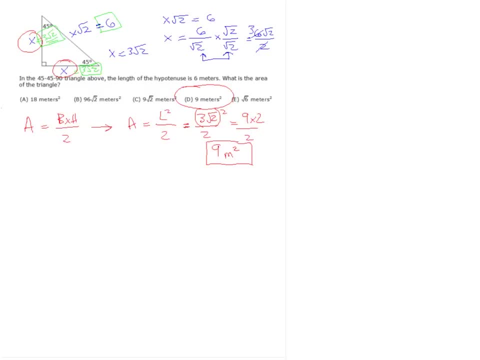 for anyone who haven't gotten to geometry, for anyone who haven't gotten to geometry yet yet. yet you know one of the first things you want. you know one of the first things you want. you know one of the first things you want to do: to do. to do is you probably want to go through, and 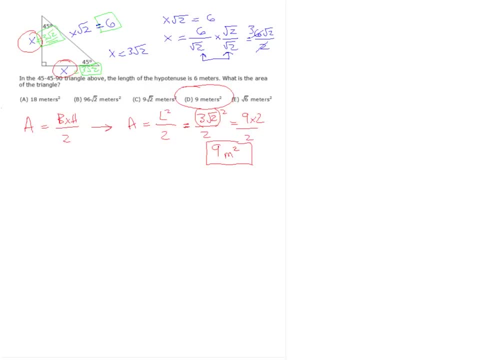 is you probably want to go through, and is you probably want to go through and you probably want to memorize? you probably want to memorize, you probably want to memorize formulas, and you know, for those of you, formulas, and you know, for those of you formulas, and you know, for those of you who don't know this, 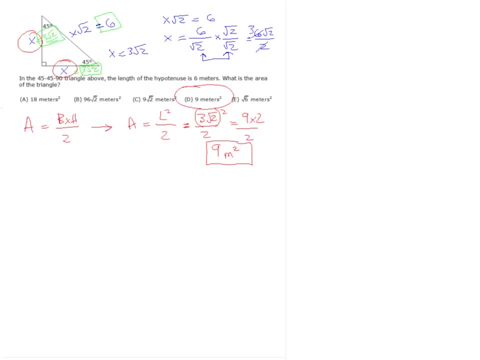 who don't know this, who don't know this? you know, on our new website, which is, you know, on our new website, which is coming out very soon, coming out very soon, coming out very soon, we are going to be giving everyone. we are going to be giving everyone. 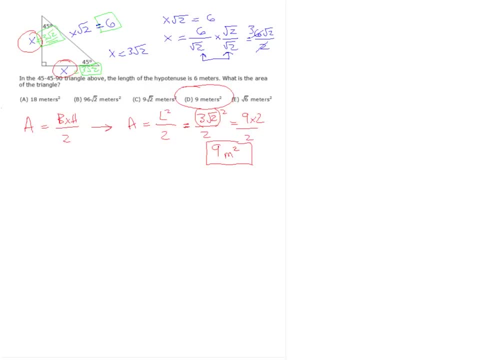 we are going to be giving everyone opportunity within opportunity within opportunity, within their own student center, to have access their own student center, to have access their own student center, to have access to all of the must knows now, to all of the must knows now, to all of the must knows now. what's so powerful about that is if you 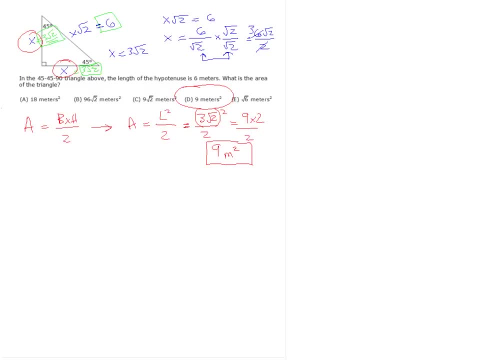 what's so powerful about that is if you. what's so powerful about that is if you go to a chapter like geometry. go to a chapter like geometry, go to a chapter like geometry, all of those must knows will be there. all of those must knows will be there. 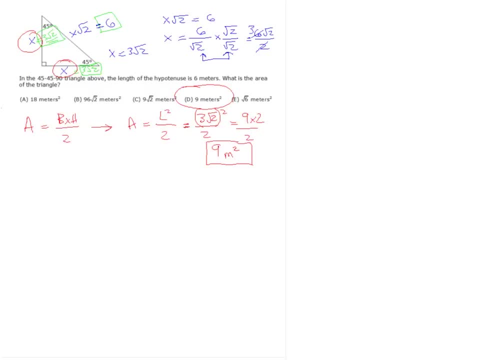 all of those, must knows, will be there for you, which basically are going to for you, which basically are going to for you, which basically are going to contain all the formulas you need to know, contain all the formulas you need to know, contain all the formulas you need to know, and you can get those guys memorized. 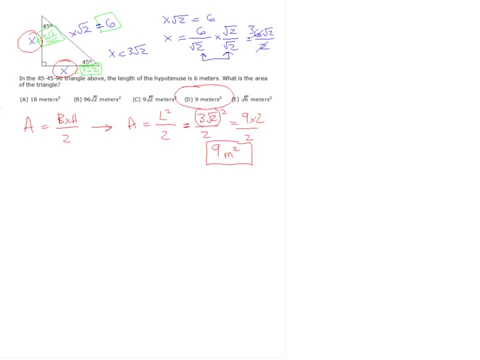 and you can get those guys memorized. and you can get those guys memorized right away. and then, if you want to right away, and then if you want to right away, and then if you want to circle back and read the chapter, because circle back and read the chapter? because 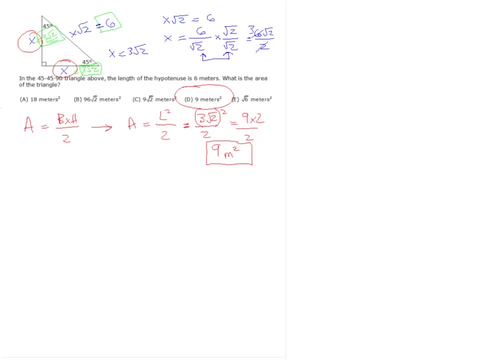 circle back and read the chapter, because the more formulas you have down, the more formulas you have down. the more formulas you have down for sure, 110 the easier. all this is for sure. 110 the easier. all this is for sure, 110 the easier all this is. so, with that said, scott, i will let you. 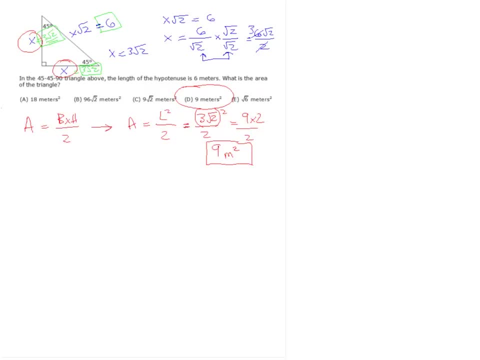 so with that said scott, i will let you. so, with that said scott, i will let you get into some more advanced stuff. get into some more advanced stuff. get into some more advanced stuff. and, uh, you can take it away, i'll pass. and uh, you can take it away, i'll pass. 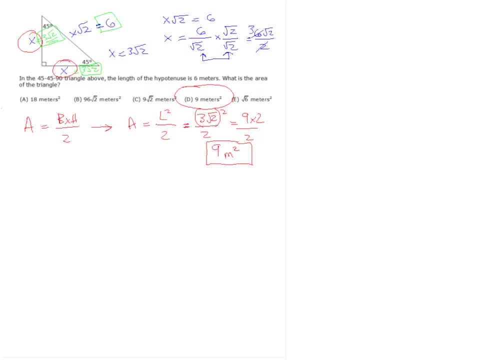 and, uh, you can take it away. i'll pass you the ball right here. all right, you should be good. good to go. all right, you should be good. good to go. all right, you should be good. good to go. you sound, you sound good and audio is you sound, you sound good and audio is. 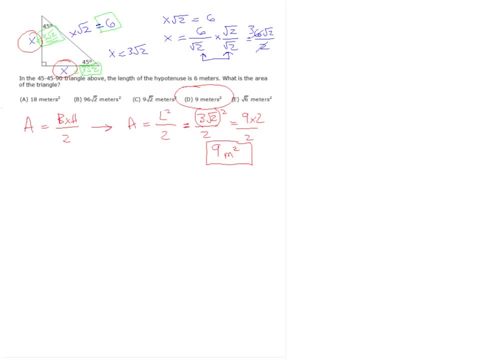 you sound, you sound good and audio is good, okay, good, great, good, okay, good, great, good, okay, good, great. hey guys, thanks for coming tonight and hey guys thanks for coming tonight and hey guys thanks for coming tonight. and jeff thanks for uh doing the first part. jeff thanks for uh doing the first part. 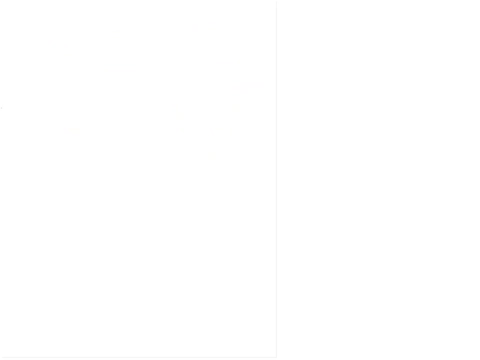 jeff, thanks for, uh, doing the first part of the webinar. as you can tell, that's of the webinar. as you can tell, that's of the webinar. as you can tell that's pretty sick, but pretty sick, but pretty sick, but did a great job. um, so what? we're going. 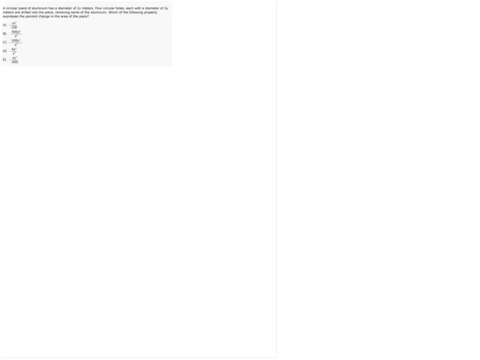 did a great job, um. so what we're going did a great job, um. so what we're going to do is don't start in this problem yet to do is don't start in this problem, yet to do is don't start in this problem yet, um, you know, as jeff said, you know. 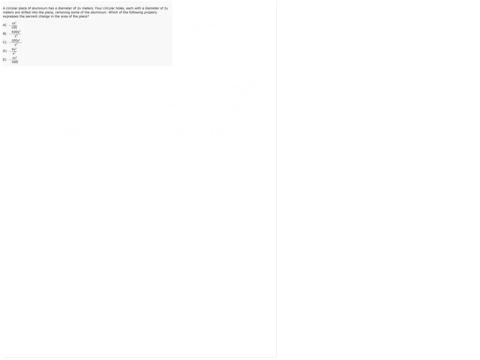 um, you know, as jeff said, you know. um, you know, as jeff said, you know, geometry is so varied and we'll end up. geometry is so varied and we'll end up. geometry is so varied and we'll end up likely doing, likely doing, likely doing. you know, probably 10 webinars in. 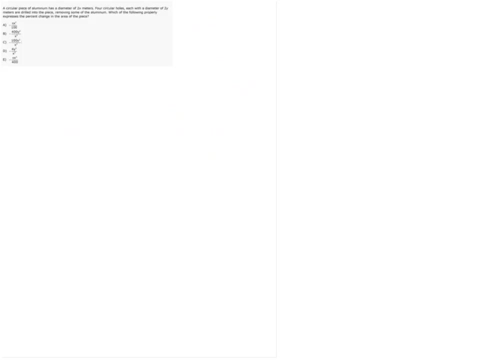 you know probably 10 webinars in. you know probably 10 webinars in geometry. there's no way to cover geometry. there's no way to cover geometry. there's no way to cover everything tonight, but i'm going to everything tonight, but i'm going to. 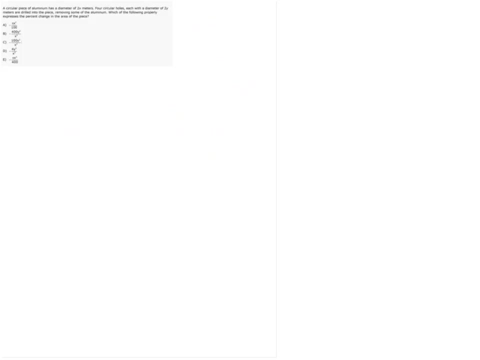 everything tonight, but i'm going to cover a bunch of uh high value stuff for cover. a bunch of uh high value stuff for cover, a bunch of uh high value stuff for the next half hour as well, the next half hour as well, the next half hour as well. um, what i'm going to try and do is 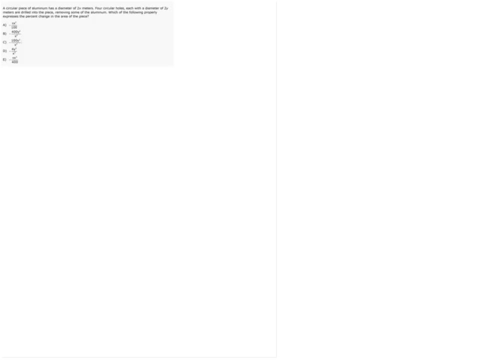 um, what i'm going to try and do is, um, what i'm going to try and do is integrate in a bunch of concepts that integrate in a bunch of concepts that integrate in a bunch of concepts that you, you, you know, if you've been playing around, 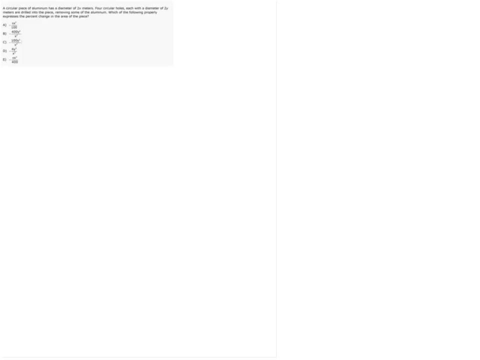 you know if you've been playing around. you know if you've been playing around geometry questions. you've seen this geometry questions. you've seen this- geometry questions. you've seen this stuff. if you have not been playing stuff, if you have not been playing stuff, if you have not been playing around geometry questions, 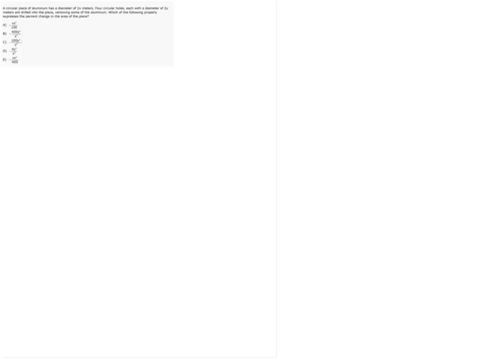 around geometry questions, around geometry questions. um, you may not expect all of these, um. you may not expect all of these, um, you may not expect all of these topics to be rolled up together. topics to be rolled up together, topics to be rolled up together. but let's give it a whirl, so we'll do. 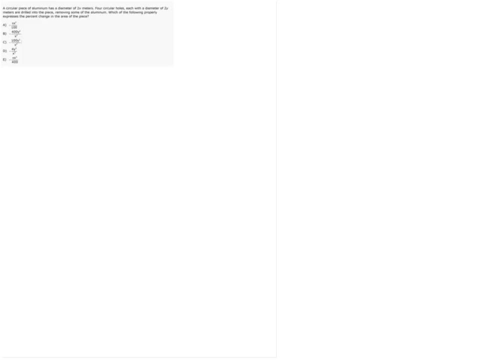 but let's give it a whirl, so we'll do. but let's give it a whirl, so we'll do a little bit more difficult. so we'll do a little bit more difficult, so we'll do a little bit more difficult. so we'll do about two and a half minutes per problem. 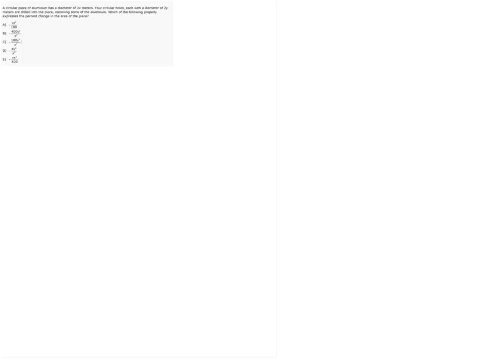 about two and a half minutes per problem. about two and a half minutes per problem. and uh, why don't we start in this first? and uh, why don't we start in this first? and uh, why don't we start in this first? guy now. guy now. guy now. yeah, good, 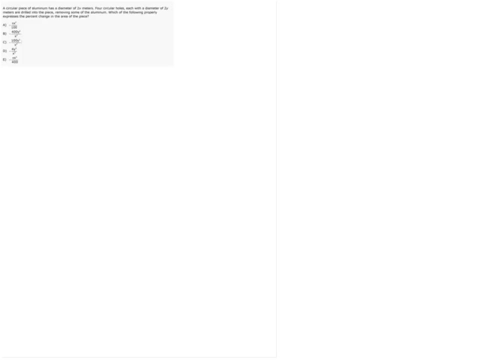 yeah, yeah, yeah, yeah, yeah, hey guys, i just reposted this. uh, hey guys, i just reposted this. uh, hey guys, i just reposted this. uh, question, question, question, question. okay guys, so that was a little bit of. okay guys, so that was a little bit of. 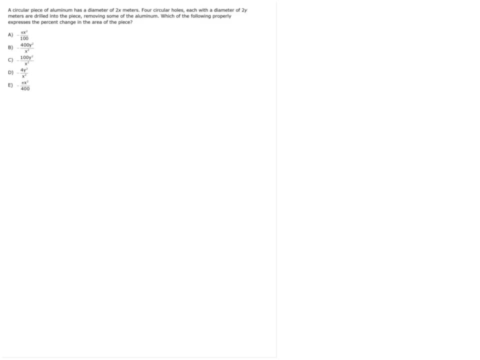 okay, guys, so that was a little bit of extra time there, so let's go over this extra time there. so let's go over this extra time there, so let's go over this together, together, together. so what we have is: we have a circular. so what we have is: we have a circular. 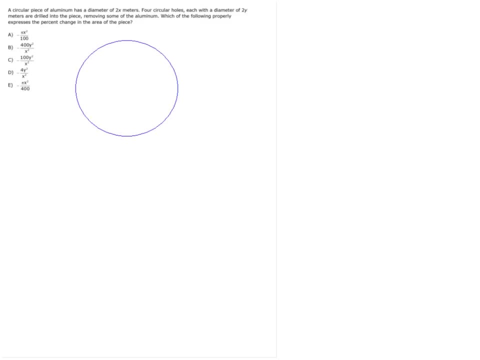 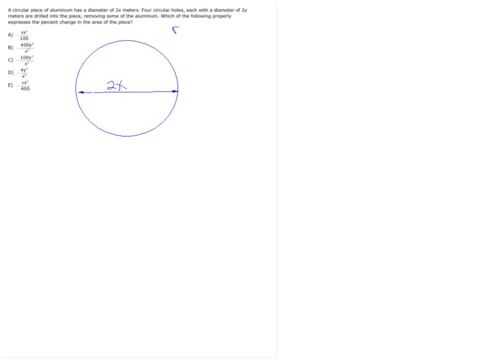 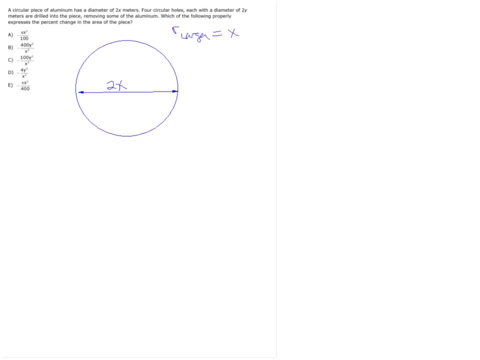 larger circle is just x meters right. larger circle is just x meters right, because the radius is obviously half of, because the radius is obviously half of, because the radius is obviously half of the, the, the diameter. so what that means is that diameter. so what that means is that 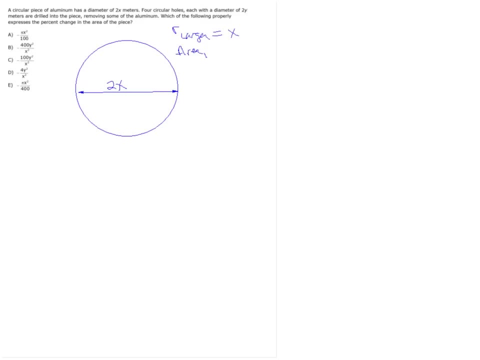 diameter. so what that means is that the area of the larger circle, you know area is of the larger circle. you know area is of the larger circle. you know area is equal to pi r squared, equal to pi r squared, equal to pi r squared. so if our radius is x, 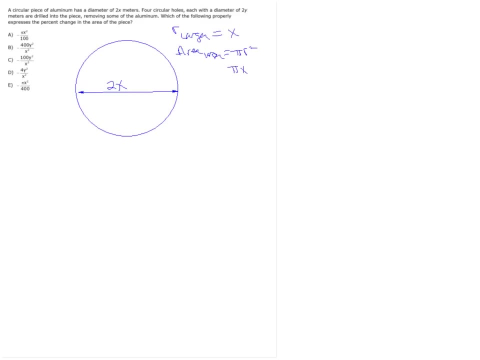 so if our radius is x. so if our radius is x, then the area is equal to pi times x. then the area is equal to pi times x, then the area is equal to pi times x squared or the larger circle here. squared or the larger circle here. 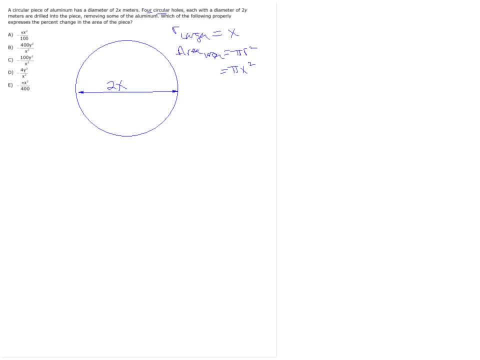 squared or the larger circle here, and then it tells us that four circular. and then it tells us that four circular. and then it tells us that four circular holes, holes, holes are drilled into this piece, so it doesn't. are drilled into this piece, so it doesn't. 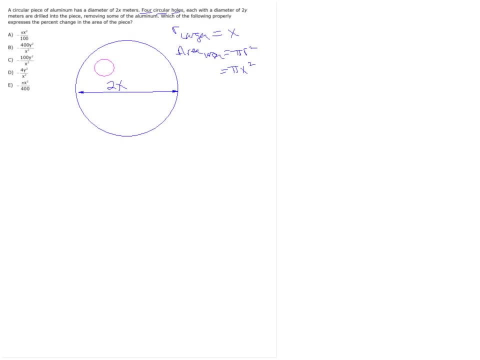 are drilled into this piece. so it doesn't really matter where they're drilled, but really matter where they're drilled, but really matter where they're drilled. but at some point, you know four, at some point you know four, at some point you know four, circular holes are drilled into this. 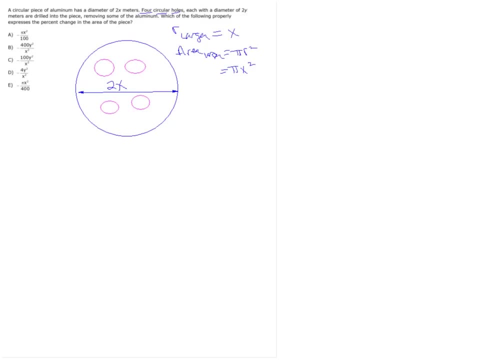 circular holes are drilled into this, circular holes are drilled into this circular piece of metal, circular piece of metal, circular piece of metal. and it says that each, and it says that each, and it says that each of these little circles has a diameter, of these little circles has a diameter. 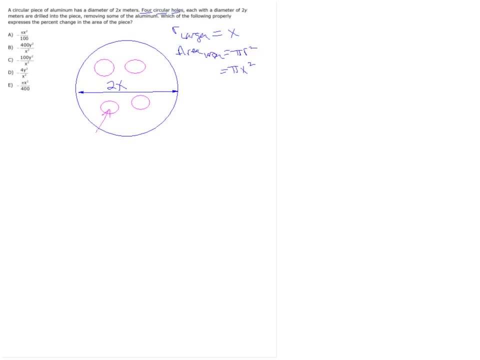 of these little circles has a diameter of two y meters, right? so the of two y meters, right, so the of two y meters, right, so the diameter of each of these guys is equal. diameter of each of these guys is equal. diameter of each of these guys is equal to two y meters. okay, 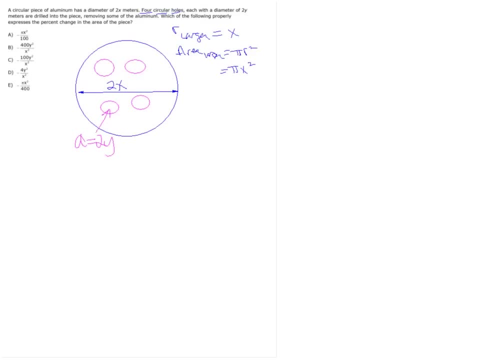 to two y meters. okay, to two y meters, okay. so if you think about what that means, so, if you think about what that means, so if you think about what that means, it means that the radius of each of the it means that the radius of each of the 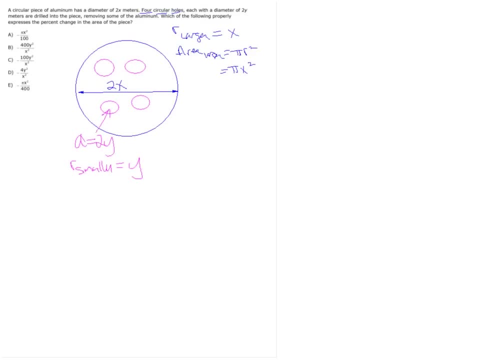 it means that the radius of each of the smaller circles is simply equal to y. smaller circles is simply equal to y. smaller circles is simply equal to y. meters. right because we know that, the meters. right because we know that the meters. right because we know that the radius is going to be half of the 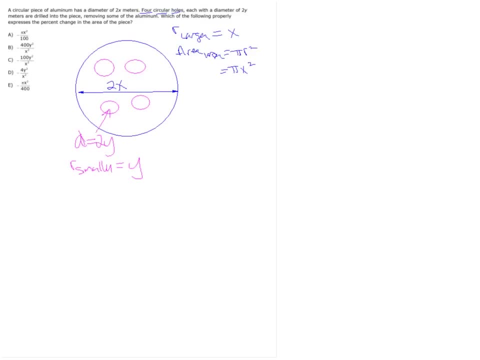 radius is going to be half of the radius is going to be half of the diameter. okay, so far so good. okay, so far so good. okay, so far, so good. so, if you think about it, we're removing so. if you think about it, we're removing. so, if you think about it, we're removing those four circular holes. 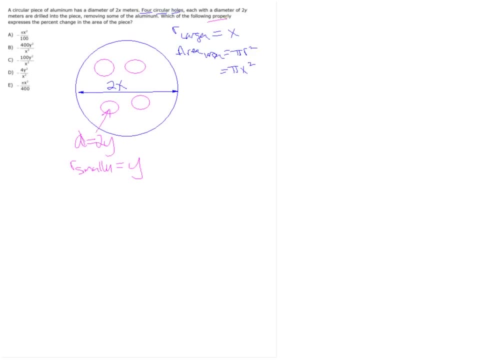 those four circular holes, those four circular holes, and we want to know which of the and we want to know which of the and we want to know which of the following properly expresses: following: properly expresses following: properly expresses: percent change: percent change, percent change of the area of the piece: 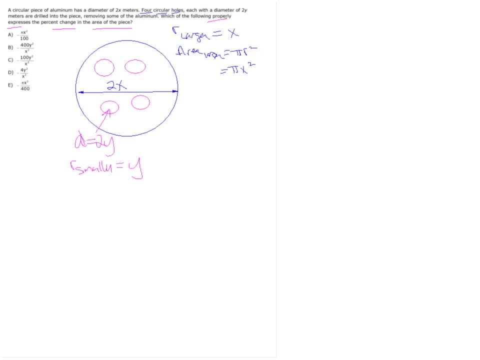 of the area of the piece, of the area of the piece. and to do this, we have to of course be, and to do this, we have to of course be, and to do this we have to of course be familiar with percent change, and it's a familiar with percent change, and it's a 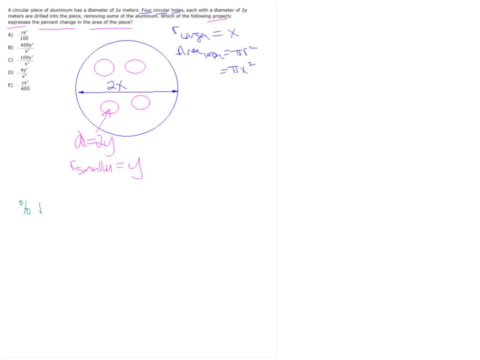 familiar with percent change and it's a really simple equation, the really simple equation, the really simple equation: the percent change and of course the percent change and of course the percent change and of course the triangle means change. in so percent triangle means change. in so percent triangle means change. in so percent change is the final value. 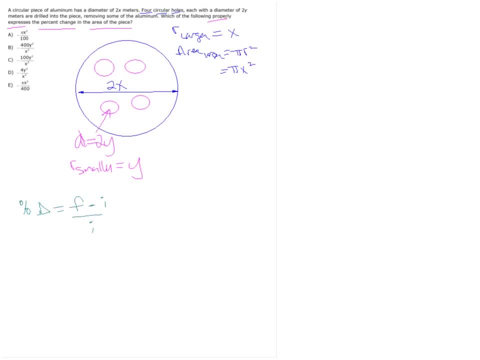 change is the final value. change is the final value minus the initial value, minus the initial value, minus the initial value, divided by the initial value, divided by the initial value, divided by the initial value, all multiplied by a hundred, all multiplied by a hundred, all multiplied by a hundred. okay, so if we're looking for the percent, 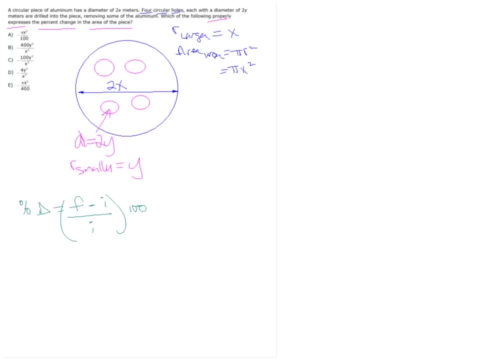 okay. so if we're looking for the percent, okay. so if we're looking for the percent, change in the area of the piece, change in the area of the piece, change in the area of the piece. we need to have the final area after the. we need to have the final area after the. 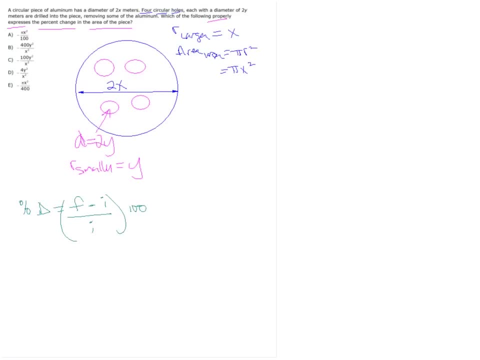 we need to have the final area after the pink holes are drilled out. pink holes are drilled out, pink holes are drilled out, and the initial area, which is just the, and the initial area, which is just the, and the initial area, which is just the area of the large blue circle prior to. 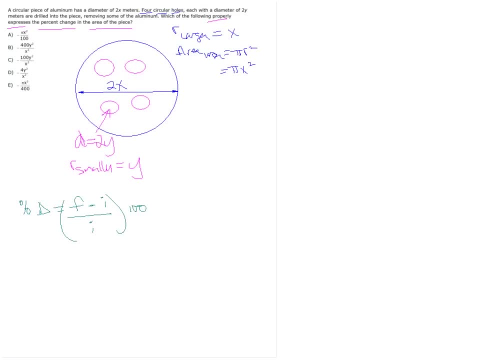 area of the large blue circle. prior to area of the large blue circle, prior to us removing those little pink circles, us removing those little pink circles, us removing those little pink circles, okay. so, if you think about it, what's the okay? so, if you think about it, what's the? 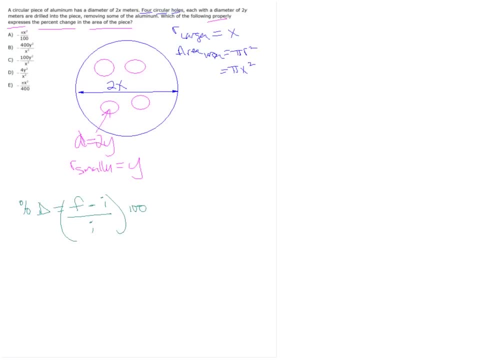 okay. so, if you think about it, what's the area that we remove, area that we remove, area that we remove? well, there are four circles. well, there are four circles. well, there are four circles, right, four little circles, right, four little circles, right, four little circles, and each of those guys have an area. 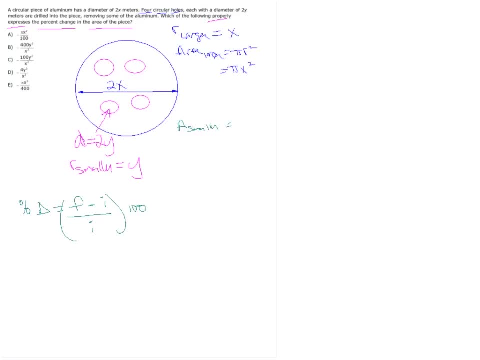 and each of those guys have an area, and each of those guys have an area. area smaller, area smaller, area smaller- each of those guys have an area of. each of those guys have an area of each of those guys have an area of pi pi pi y squared. 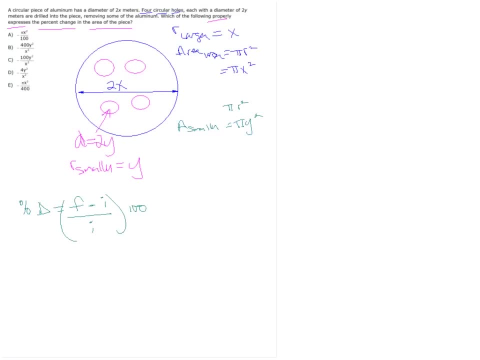 y squared, y squared right, because, remember, area is simply pi right, because, remember, area is simply pi right, because remember, area is simply pi r squared, r squared, r squared. and we said that the radius of the and we said that the radius of the and we said that the radius of the smaller circles is y. 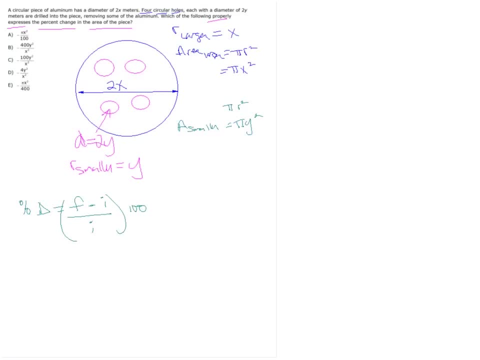 smaller circles is y, smaller circles is y. so what that means is: the area is pi. so what that means is: the area is pi. so what that means is the area is pi times y squared times y squared times y squared. but if you think about it, there are four. 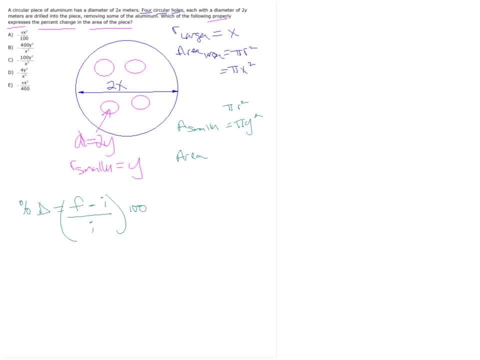 but if you think about it, there are four, but if you think about it, there are four of them, of them, of them. so the area, so the area, so the area removed, removed, removed, would simply be four equal to four, would simply be four equal to four would simply be four equal to four times pi y squared right, just to make. 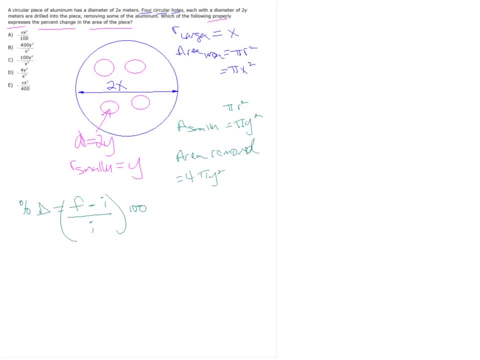 times pi y squared right, just to make times pi y squared right, just to make sure everyone's following along, sure, everyone's following along, sure, everyone's following along. so if each of the smaller, so if each of the smaller, so if each of the smaller, so if each of the circles. 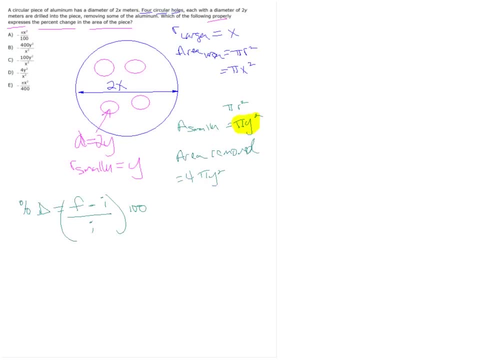 so if each of the circles, so if each of the circles have an area of pi y squared, have an area of pi y squared, have an area of pi y squared, and if you have four of them and they're, and if you have four of them and they're, 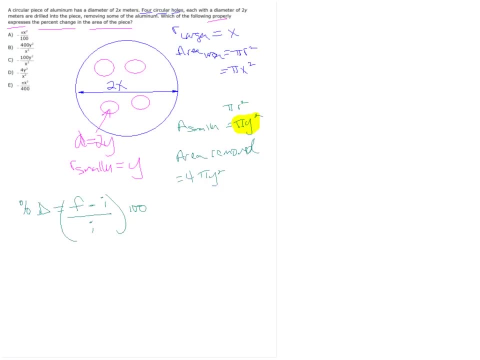 and if you have four of them and they're all the same, well, you're removing a all the same. well, you're removing a all the same. well, you're removing a total area, total area. total area of four pi y squared from the big blue, of four pi y squared from the big blue. 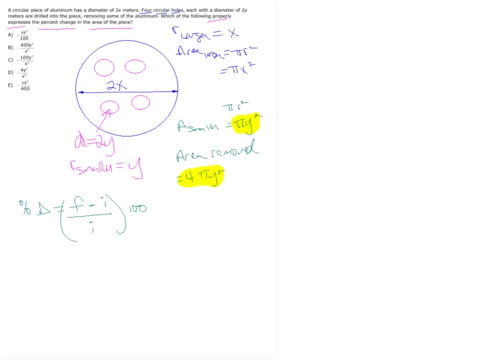 of four, pi, y, squared from the big blue circle. okay, so then with that information we can okay. so then, with that information we can okay. so then with that information we can calculate the percent change, calculate the percent change, calculate the percent change. so, if you think about it, now watch cap. 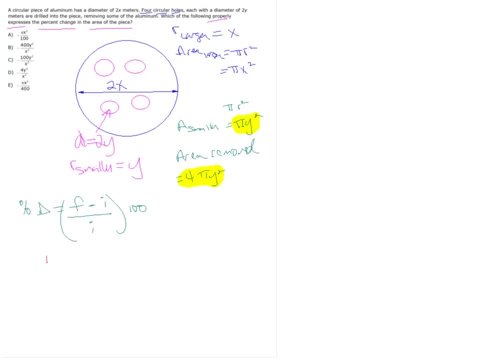 so if you think about it now, watch cap. so if you think about it now, watch cap carefully here. so the final value is the carefully here. so the final value is the carefully here. so the final value is the initial, initial, initial value of the blue circle, the initial area. 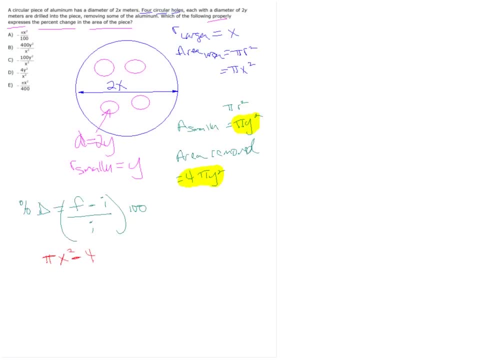 value of the blue circle. the initial area value of the blue circle: the initial area of the blue circle, of the blue circle, of the blue circle, minus the four pi y squared, which is the minus the four pi y squared, which is the minus the four pi y squared, which is the area we have. 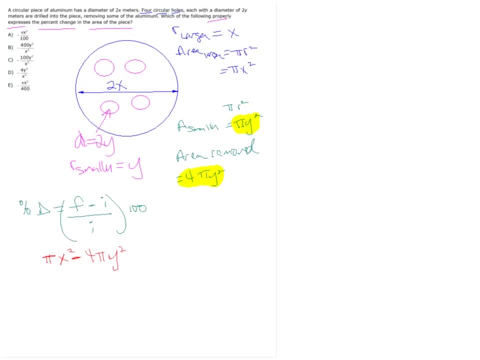 area we have, area we have removed, removed, removed- right those little pink circles, right those little pink circles, right those little pink circles minus. so here's the initial value minus. so here's the initial value minus. so here's the initial value. initial value is pi. initial value is pi. 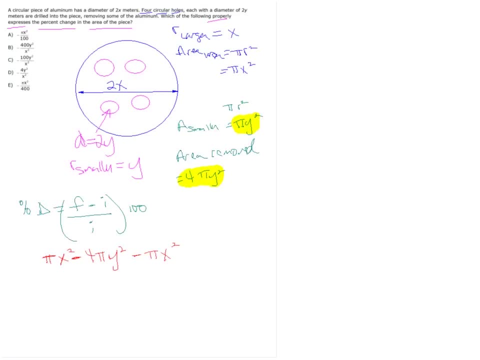 initial value is pi x squared right. that's just the x squared right. that's just the x squared right. that's just the initial area of the blue circle. initial area of the blue circle, initial area of the blue circle, divided by the initial value. divided by the initial value. 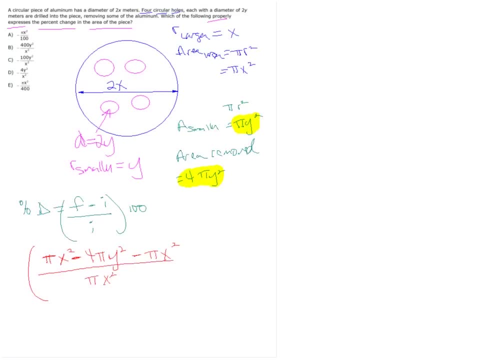 divided by the initial value of the area of the blue circle, of the area of the blue circle, of the area of the blue circle, and of course this is multiplied by, and of course this is multiplied by, and of course this is multiplied by 100.. 100. 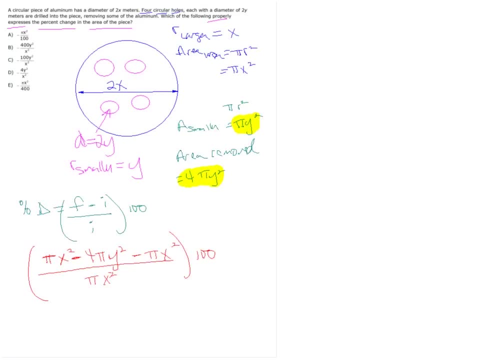 100.. you guys, of course, obviously you're, you guys, of course, obviously you're. you guys, of course obviously you're going to have to scroll down to see some, going to have to scroll down to see some going to have to scroll down to see some of it. 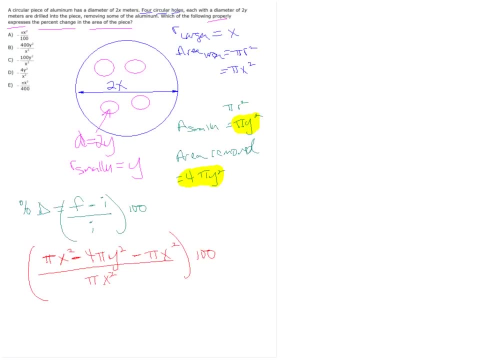 of it, of it. so now we need to simplify this, and it's so, now we need to simplify this, and it's so now we need to simplify this, and it's just going back to the stuff that you just going back to, the stuff that you just going back to the stuff that you know we always preach, which is a 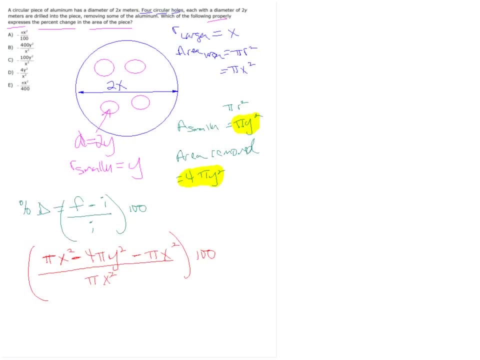 know we always preach, which is a know we always preach, which is a. you need to capitalize on every. you need to capitalize on every. you need to capitalize on every factorable opportunity that you can, factorable opportunity that you can, factorable opportunity that you can. and you can notice here that in the 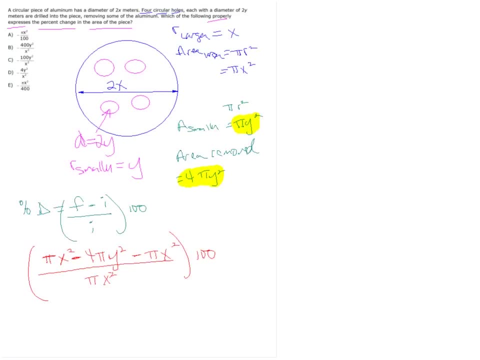 and you can notice here that in the, and you can notice here that in the numerator there are three terms. numerator, there are three terms numerator, there are three terms and each of these terms contains a pi and each of these terms contains a pi and each of these terms contains a pi. so what we can and should do is factor. 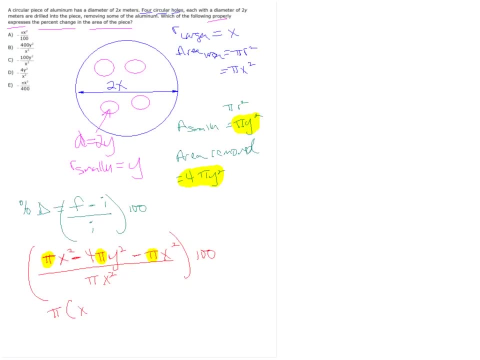 so what we can and should do is factor. so what we can and should do is factor out that pi, out that pi, out that pi, and we'll be left with x squared, and we'll be left with x squared, and we'll be left with x squared minus 4 y squared. 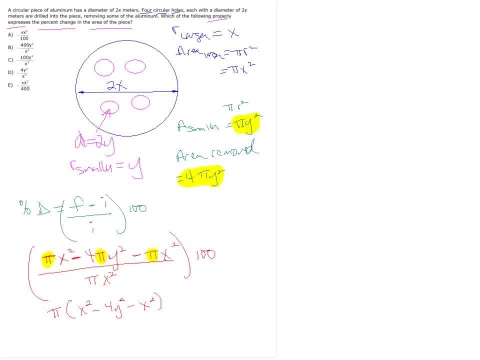 minus 4 y squared minus 4 y squared. minus x squared. minus x squared. minus x squared over over over pi x squared. pi x squared, pi x squared, and of course this is still multiplied by, and of course this is still multiplied by, and of course this is still multiplied by 100. 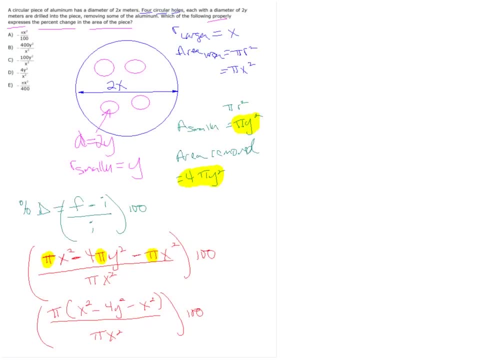 100 and of course, the benefit to factoring out and of course, the benefit to factoring out and, of course, the benefit to factoring out that that that pi was. we can see that this pi will pi was. we can see that this pi will pi was. we can see that this pi will cancel with this pi. 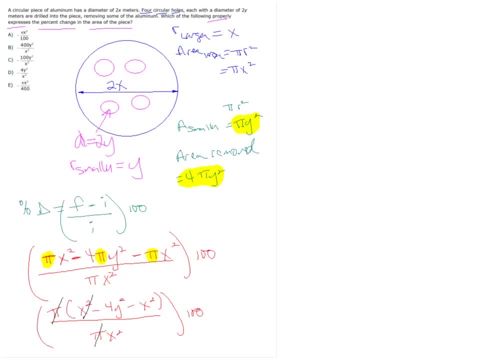 cancel with this pi, cancel with this pi. and then in the numerator in those, and then in the numerator in those, and then in the numerator in those, parentheses. we see we have x squared and parentheses. we see we have x squared and parentheses. we see we have x squared and minus x squared and those guys cancel. 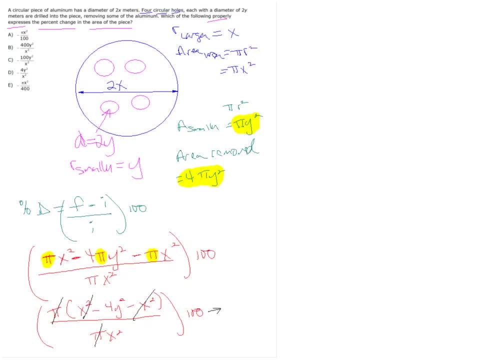 minus x squared and those guys cancel. minus x squared and those guys cancel. i'm going to have to write small over. i'm going to have to write small over. i'm going to have to write small over here, here, here, but we're basically left with, but we're basically left with. 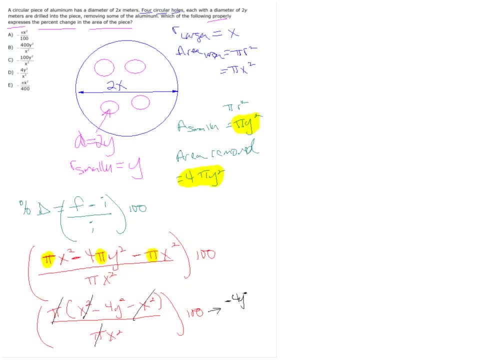 but we're basically left with minus, minus, minus. 4 y squared 4 y squared 4 y squared over x squared over x squared over x squared times: 100 right times, 100 right times, 100 right, which gives us minus. which gives us minus. which gives us minus 400. 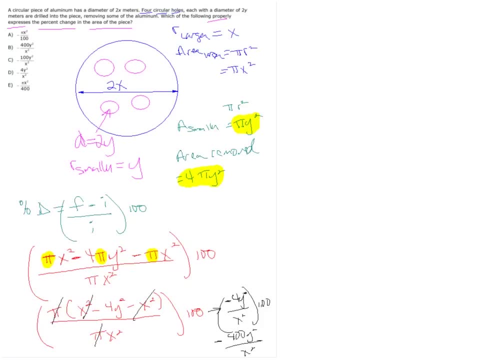 400, 400. y squared, y squared, y squared over x squared over, x squared over x squared. and at this point, there's nothing more and at this point, there's nothing more, and at this point, there's nothing more that we can simplify, that we can simplify. 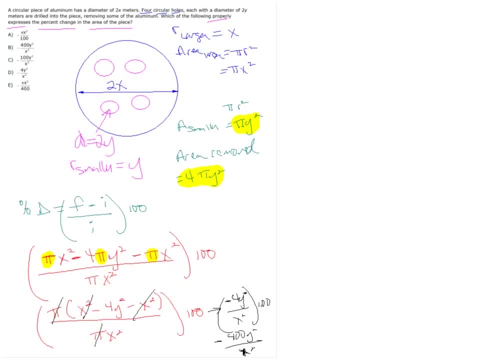 that we can simplify and let's hope that that answer choice is and let's hope that that answer choice is and let's hope that that answer choice is up there up there up there. yes, it is so, that's answer choice b. yes, it is so, that's answer choice b. 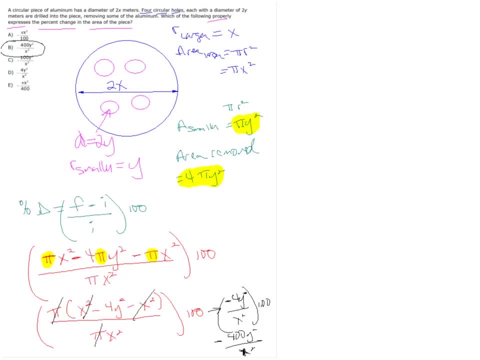 yes, it is so. that's answer choice b: as in boy, as in boy, as in boy, so so so this is a really good problem, um a. this is a really good problem, um a. this is a really good problem, um a, because it's pretty challenging. because it's pretty challenging. 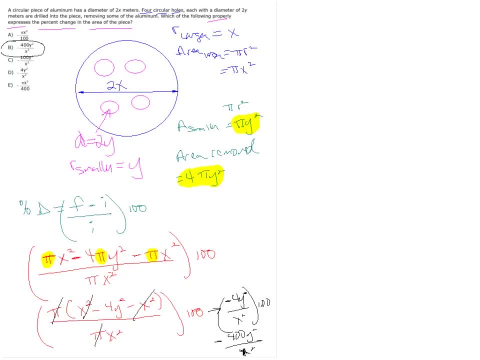 because it's pretty challenging, and b because it integrates a lot of, and b because it integrates a lot of, and b because it integrates a lot of ideas. right, we had an area of the ideas. right, we had an area of the ideas. right, we had an area of the circle we had to sort of logically 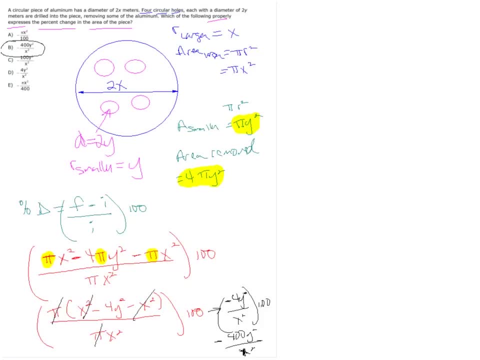 circle. we had to sort of logically circle. we had to sort of logically figure out the total area removed and figure out the total area removed, and figure out the total area removed. and then we had to integrate. then we had to integrate, then we had to integrate in the idea of percent change. and you're. 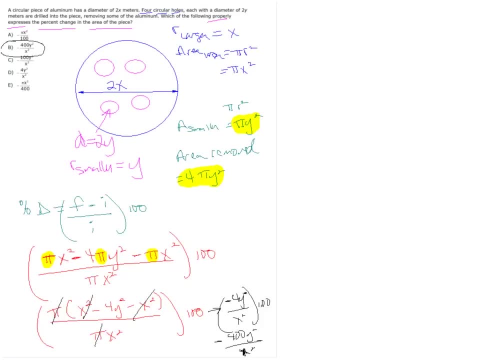 in the idea of percent change, and you're in the idea of percent change and you're going to see a lot of medium to going to see a lot of medium to going to see a lot of medium to difficulty map probably do just this. difficulty map probably do just this. 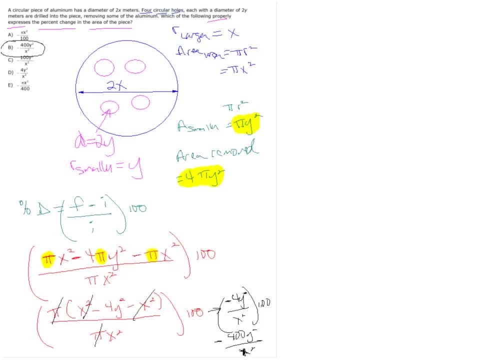 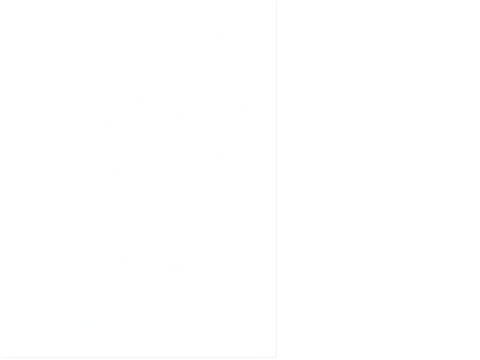 difficulty map probably do just this. so give everybody a minute. so give everybody a minute. so give everybody a minute, catch up any notes on that, catch up any notes on that, catch up any notes on that and we'll do another one. okay, okay, okay. so, keeping with our theme of 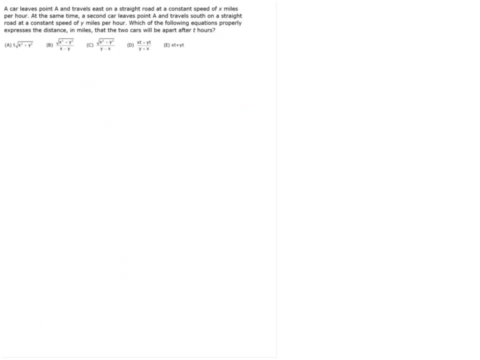 so keeping with our theme of so keeping with our theme of integrating in different topics. integrating in different topics, integrating in different topics. what i'm going to do is we're going to. what i'm going to do is we're going to. what i'm going to do is we're going to integrate in a rate equation with the. 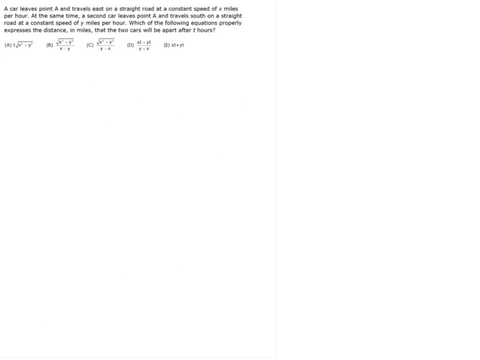 integrate in a rate equation with the. integrate in a rate equation with the geometry problem here. geometry problem here. geometry problem here. so the key to anywhere problem is a. so the key to anywhere problem is a. so the key to anywhere problem is a. take it step by step and b. 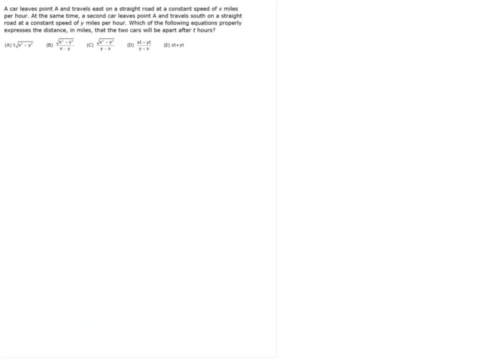 take it step by step and b. take it step by step and b with geometry. make yourself a drawing with geometry. make yourself a drawing with geometry. make yourself a drawing. a picture is worth more than a thousand. a picture is worth more than a thousand. a picture is worth more than a thousand words. on the test and we'll shoot for. 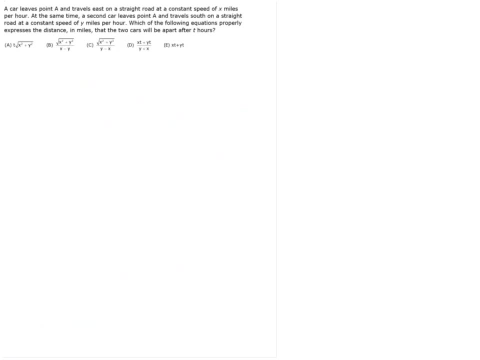 words on the test and we'll shoot for words on the test and we'll shoot for about three minutes to do this, guys, about three minutes to do this, guys, about three minutes to do this, guys, let's start our clocks now. let's start our clocks now. 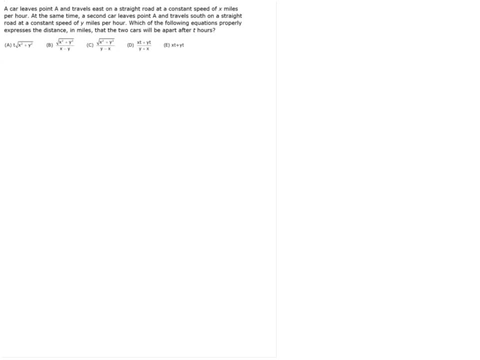 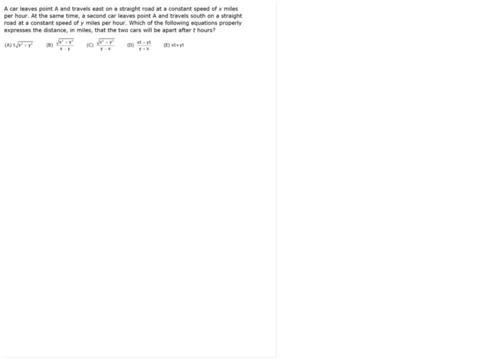 so we have a car at least point a, and it. so we have a car, at least point a, and it travels east on the strait, travels east on the strait, travels east on the strait road, and we know that it travels at a road and we know that it travels at a. 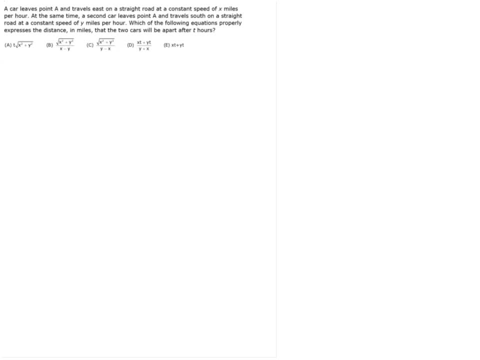 road and we know that it travels at a constant speed of x miles per hour. constant speed of x miles per hour. constant speed of x miles per hour, same time the second car leaves point a same time. the second car leaves point a same time. the second car leaves point a and it travels south on a straight road. 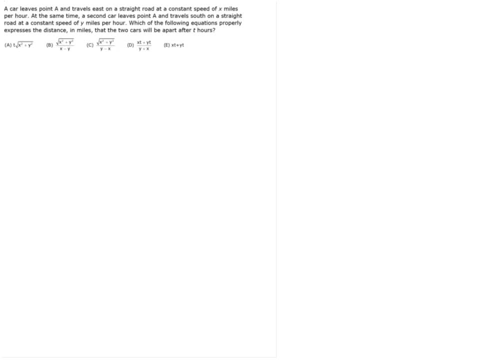 and it travels south on a straight road. and it travels south on a straight road at a constant speed of y miles per hour, at a constant speed of y miles per hour, at a constant speed of y miles per hour. so let's just diagram that out. it's. 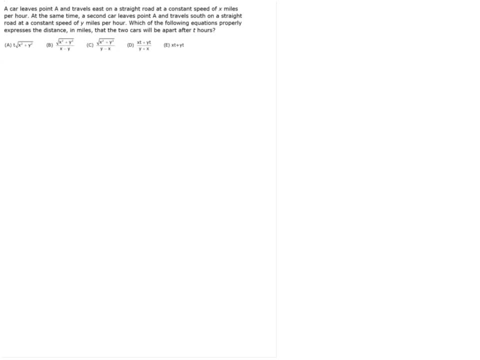 so let's just diagram that out. it's so, let's just diagram that out. it's going to become a lot clearer. so, going to become a lot clearer, so going to become a lot clearer. so let's say this, let's say this, let's say this arrow is emanating from point a and going: 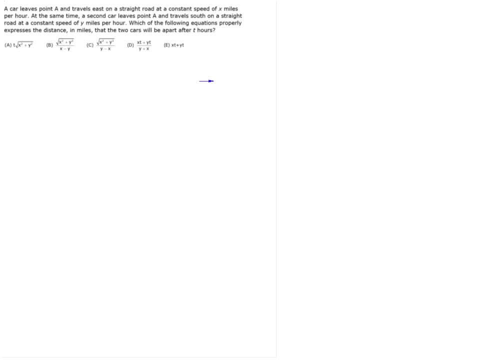 arrow is emanating from point a and going arrow is emanating from point a and going east, east, east. and this arrow is emanating from point a and this arrow is emanating from point a and this arrow is emanating from point a and going south. 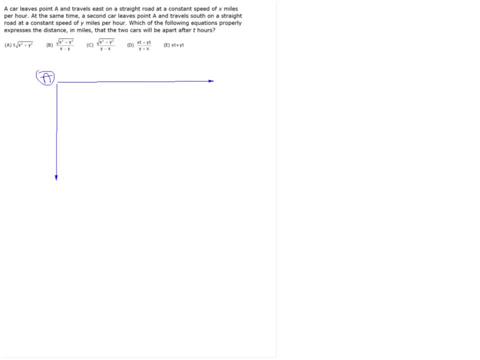 and going south and going south. right so this is our starting point, right so this is our starting point, right so this is our starting point, right here. this is a right here. this is a right here. this is a, and it says that the car that leaves a. 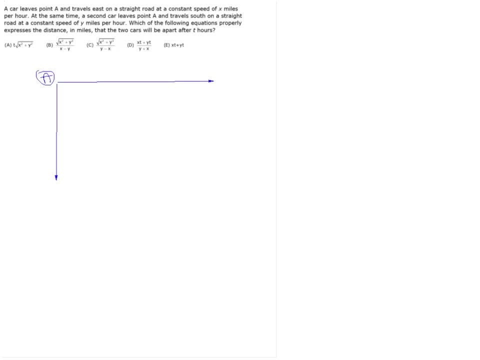 and it says that the car that leaves a. and it says that the car that leaves a travels at x miles per hour. travels at x miles per hour. travels at x miles per hour in the car that leaves a and goes south. in the car that leaves a and goes south. 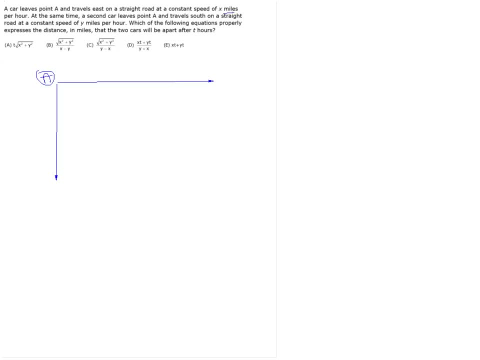 in the car that leaves a and goes south, travels at y miles per hour at least. travels at y miles per hour at least. travels at y miles per hour at least. speeds of x and y respectively. speeds of x and y respectively. speeds of x and y respectively. it says which of the following equations: 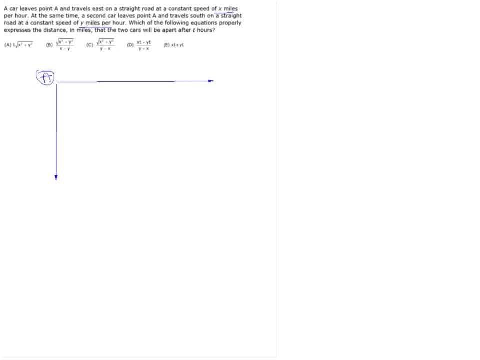 it says which of the following equations it says which of the following equations properly expresses the distance in miles? properly expresses the distance in miles. properly expresses the distance in miles. that the two cars will be apart after 50. that the two cars will be apart after 50. 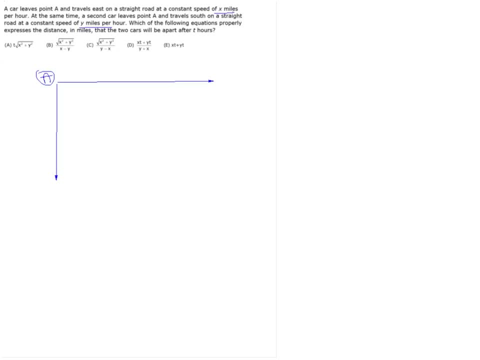 that the two cars will be apart after 50 hours. well hours, well hours. well, you know, guys, here's the biggest secret. you know, guys, here's the biggest secret. you know, guys, here's the biggest secret about math and if you can catch on to about math and if you can catch on to. 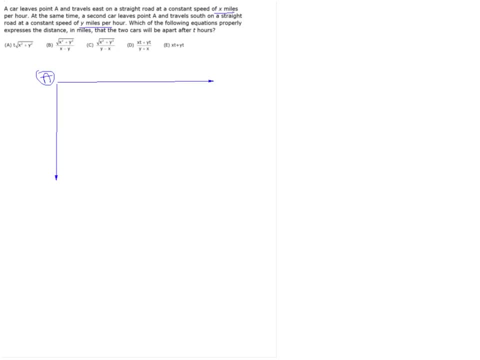 about math and if you can catch on to this, you're going to be ahead of like this. you're going to be ahead of like this. you're going to be ahead of like literally everyone in the world and literally everyone in the world and literally everyone in the world, and that's not an exaggeration. so the 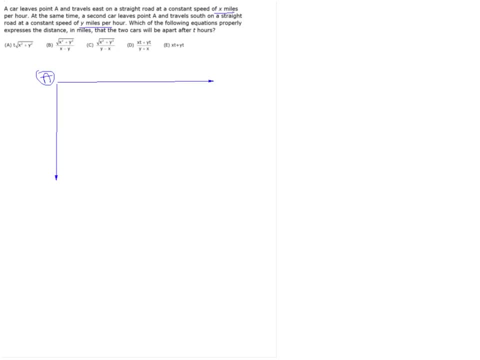 that's not an exaggeration. so the that's not an exaggeration. so the beauty about math is: no one can lie to. beauty about math is no one can lie to. beauty about math is no one can lie to you, no one can deceive you, no one can. 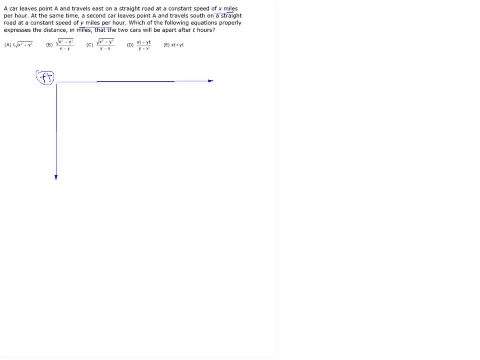 you. no one can deceive you. no one can you. no one can deceive you, no one can trick you. and you're saying, yeah right, trick you. and you're saying, yeah right, trick you. and you're saying, yeah right, that's the whole gmat, but it's not. 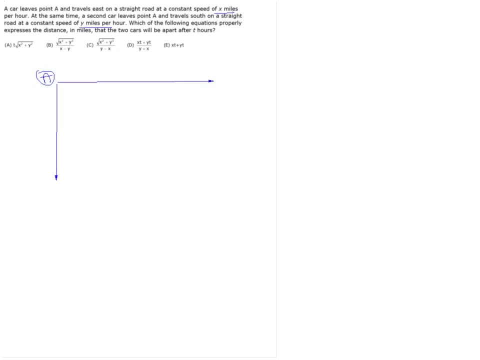 that's the whole gmat, but it's not. that's the whole gmat, but it's not right. they're only going to trick the right. they're only going to trick the right. they're only going to trick the people who haven't got the information. 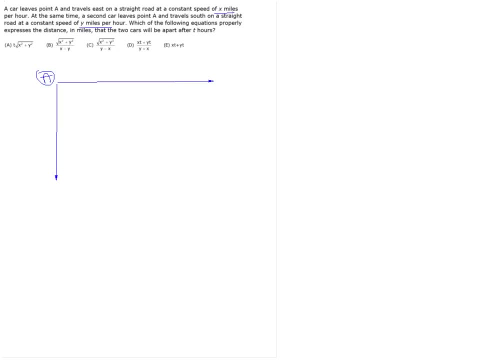 people who haven't got the information, people who haven't got the information, down, path, down, path, down path, right in all other uh disciplines, maybe right in all other uh disciplines, maybe right in all other uh disciplines, maybe with the exception of chemistry, and with the exception of chemistry, and 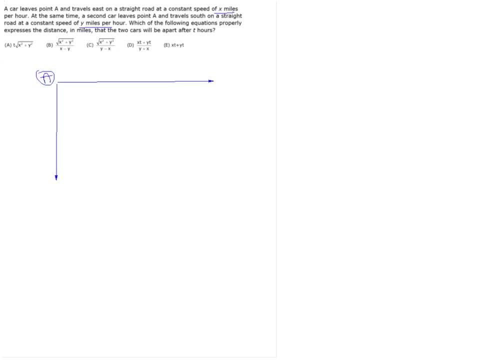 with the exception of chemistry and physics. you know things that actually physics. you know things that actually physics. you know things that actually rest upon mathematics. rest upon mathematics, rest upon mathematics. people can easily deceive other people. people can easily deceive other people. people can easily deceive other people who are unsuspecting and not saying that. 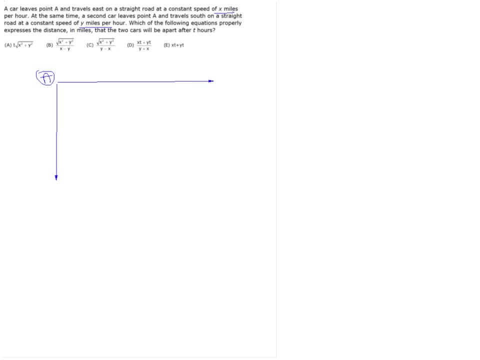 who are unsuspecting and not saying that. who are unsuspecting and not saying that people don't do that enough as well, but people don't do that enough as well. but people don't do that enough as well. but it happens to the unsuspecting people. it happens to the unsuspecting people. 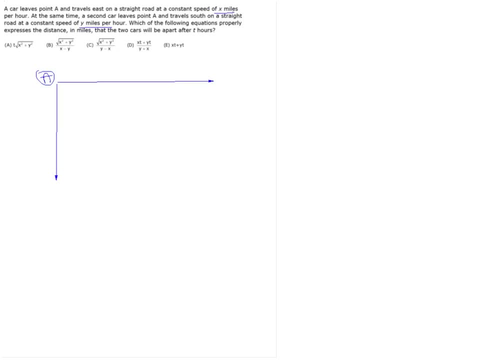 it happens to the unsuspecting people and where is all this going? and where is all this going? and where is all this going? well, in these word problems. they a well in these word problems. they a well in these word problems. they a have to give you the necessary facts. 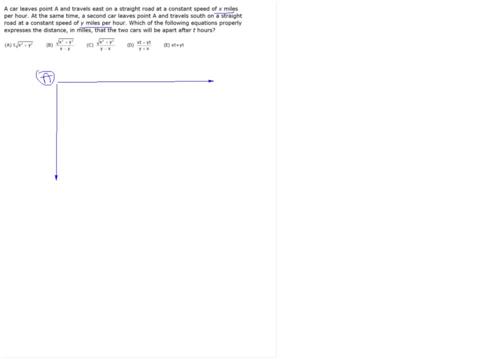 have to give you the necessary facts, have to give you the necessary facts right. how often can you say that happens right? how often can you say that happens right? how often can you say that happens in the business world, in the business world, in the business world? and b they have to actually ask you the. 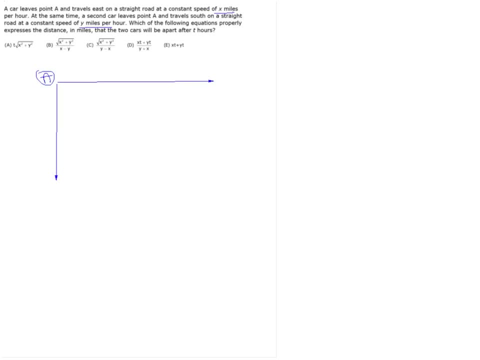 and b they have to actually ask you the and b- they have to actually ask you the question they want to know, question they want to know, question they want to know. and how often does that happen, right so? and how often does that happen, right so? and how often does that happen, right so? on a problem like this, the clues are all. 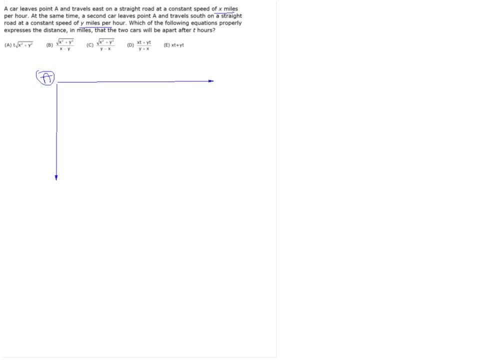 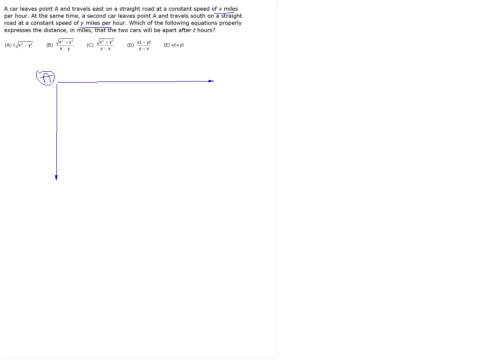 which of the following equations: which of the following equations properly expresses the distance? properly expresses the distance? properly expresses the distance in miles? well, immediately, we're talking in miles. well, immediately, we're talking in miles. well, immediately, we're talking about distance, about distance, about distance, like all we need to do is say to. 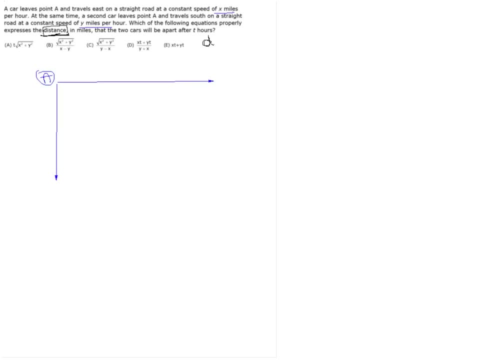 like. all we need to do is say to like. all we need to do is say to ourselves: well ourselves, well ourselves. well, distance is equal to the rate object distance is equal to the rate object distance is equal to the rate object travels multiplied by the time it takes. 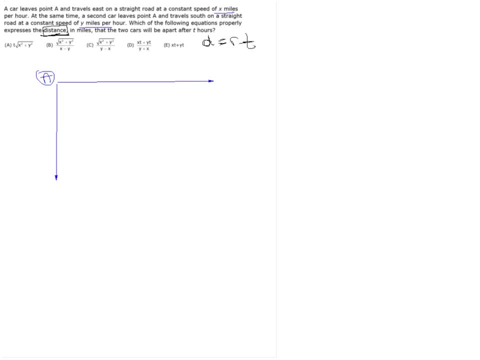 travels multiplied by the time it takes. travels multiplied by the time it takes, you know, multiplied by the traveling time, you know, multiplied by the traveling time, you know, multiplied by the traveling time. and it's that simple. and it's that simple, and it's that simple, right so, right away now, what we can say. 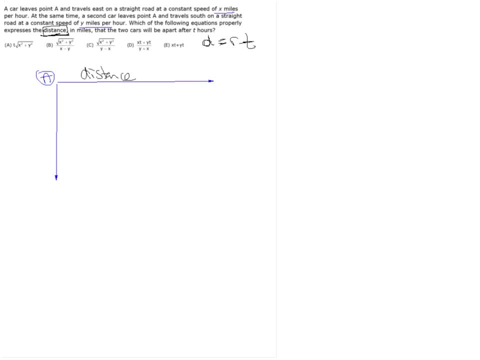 right so, right away now. what we can say, right so, right away now, what we can say is the distance. the car is the distance, the car is the distance. the car that travels east travels is equal. that travels east travels is equal. that travels east travels is equal to x? t? right, because they're asking us. 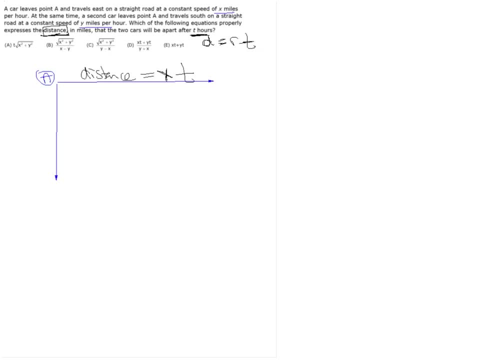 to x t right because they're asking us. to x t right because they're asking us. you know how far will the cars be apart. you know how far will the cars be apart. you know how far will the cars be apart after t hours, after t hours. 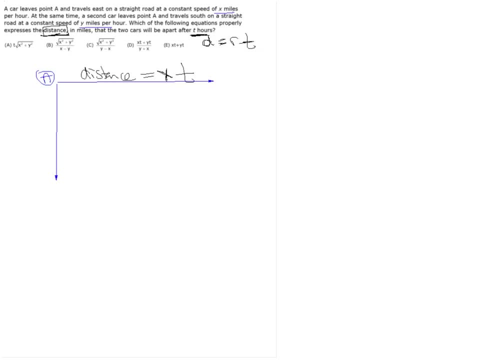 after t hours. okay, so that was a critical little piece. okay, so that was a critical little piece. okay, so that was a critical little piece of nugget i just gave you. is that in a of nugget i just gave you? is that in a of nugget i just gave you? is that in a word problem? 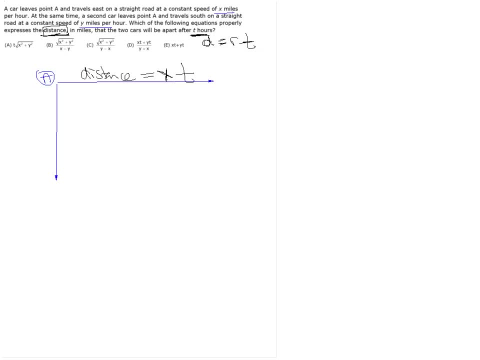 word problem, word problem: everything is there and what will be asked? everything is there and what will be asked. everything is there and what will be asked is exactly what's needed, is exactly what's needed, is exactly what's needed. there's no ambiguity going on. there's no ambiguity going on. 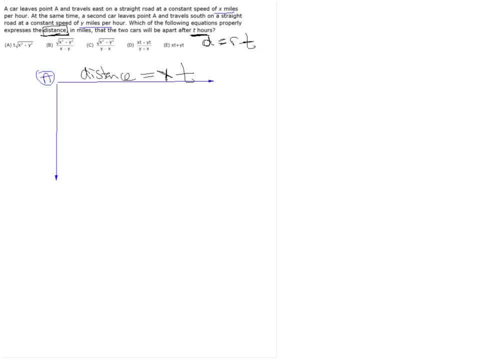 there's no ambiguity going on. okay, so the distance is x times t. okay, so the distance is x times t. okay, so the distance is x times t from a to the east, from a to the east, from a to the east, and then the distance going south. 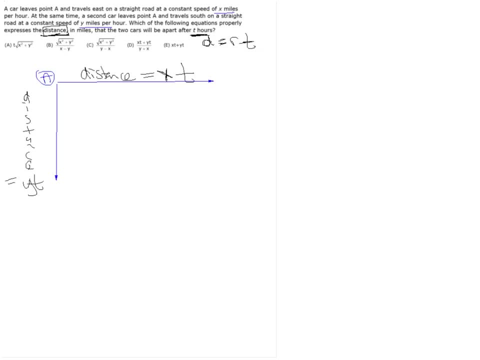 going south. going south will be equal to, will be equal to, will be equal to right x times t and y times t, right x times t and y times t, right x times t and y times t. and that's a very simple equation now. and that's a very simple equation now. 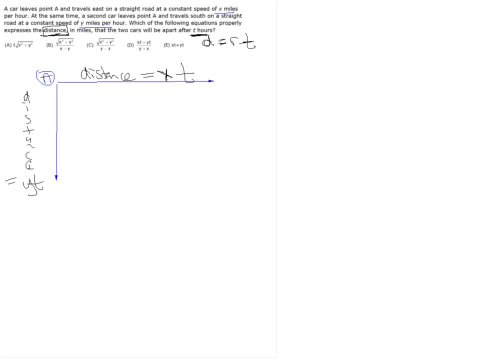 and that's a very simple equation. now, obviously you know, with all of you knew. obviously you know with all of you knew. obviously you know, with all of you knew, distance is rate times time. distance is rate times time. distance is rate times time. well, now they're asking you how far are? 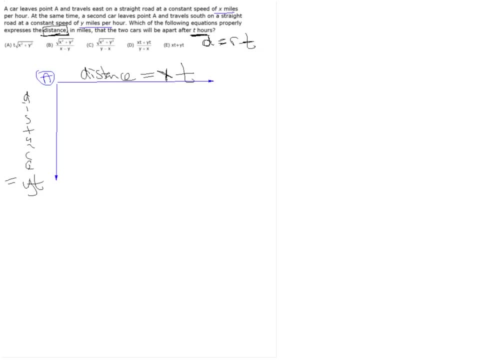 well, now they're asking you: how far are? well, now they're asking you: how far are the cars going to be apart? the cars going to be apart, the cars going to be apart. and of course, if you think about like, and of course, if you think about like. 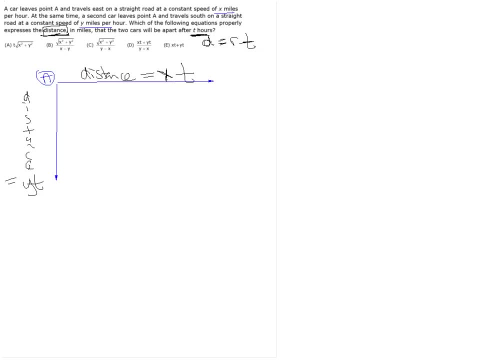 and, of course, if you think about, like the physical distance, the physical distance, the physical distance, that these cars are apart, well, it's the that these cars are apart. well, it's the that these cars are apart. well, it's the hypotenuse of a right triangle. 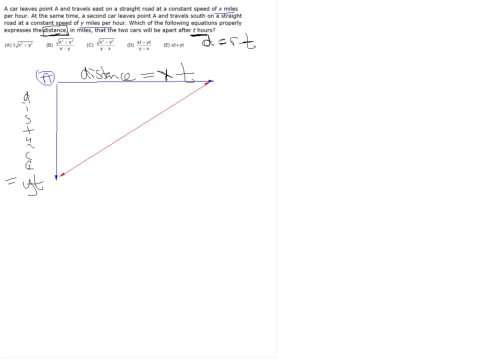 hypotenuse of a right triangle. hypotenuse of a right triangle. big surprise, right. big surprise, right. big surprise, right. okay, we know this is a triangle a right. okay, we know this is a triangle a right. okay, we know this is a triangle, a right triangle because we let one. 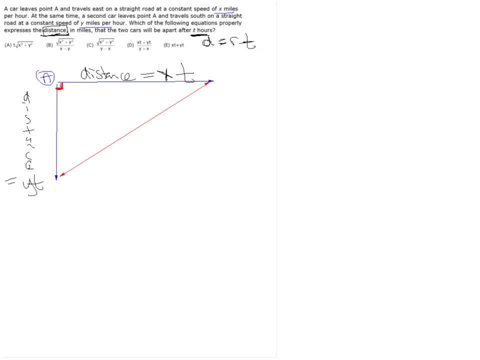 triangle. because we let one triangle, because we let one um ray emanate to the east and one ray um ray emanate to the east, and one ray um ray emanate to the east and one ray emanated to the salt. so this is by emanated to the salt, so this is by. 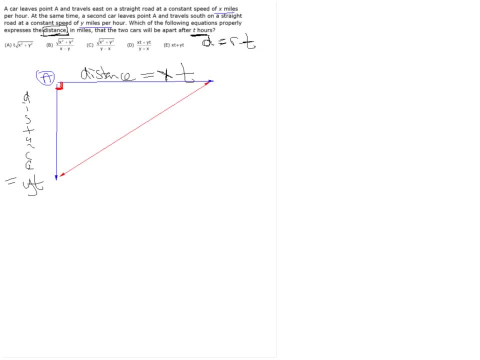 emanated to the salt. so this is, by definition, right triangle, definition, right triangle, definition, right triangle. and if we let d be this unknown, and if we let d be this unknown, and if we let d be this unknown distance, and this is where i want you to 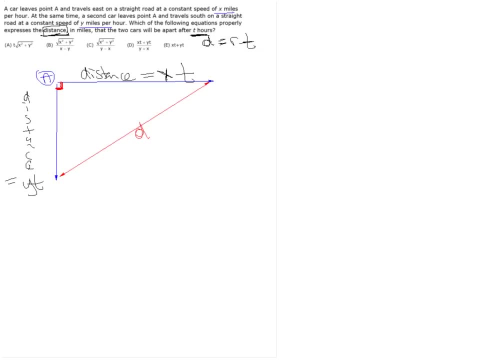 distance, and this is where i want you to distance and this is where i want you to pay careful attention, pay careful attention, pay careful attention. well, we can write an equation. well, we can write an equation. well, we can write an equation. we can say d. we can say d. 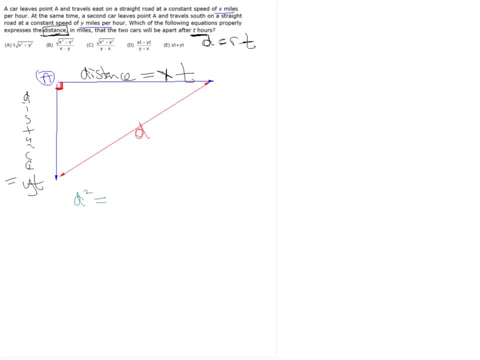 we can say: d squared by the hypotenuse squared, squared by the hypotenuse squared. squared by the hypotenuse squared is equal to the length of one, is equal to the length of one, is equal to the length of one side squared, side squared, side squared, plus the length of the other side. 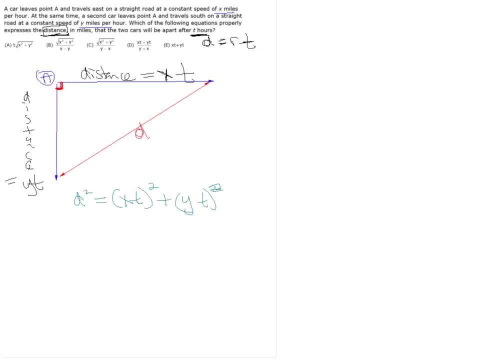 plus the length of the other side plus the length of the other side, squared, squared, squared right. so just remember, because distance right. so just remember, because distance right. so just remember, because distance is rate times time we actually is rate times time we actually is rate times time we actually algebraically let the distance of this 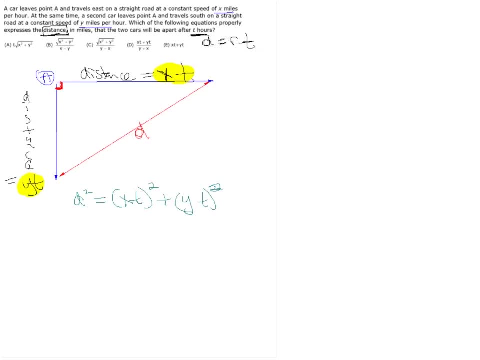 algebraically, let the distance of this. algebraically, let the distance of this line be xt, line be xt, line be xt, and we let the distance of this line be, and we let the distance of this line be, and we let the distance of this line be yt. 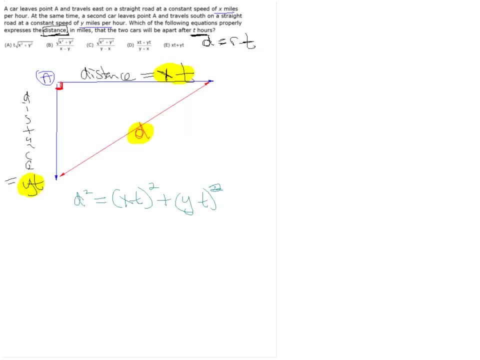 yt, yt. and if we're solving for the total, and if we're solving for the total, and if we're solving for the total distance, distance, distance- well, we can use the pythagorean theorem. well, we can use the pythagorean theorem. well, we can use the pythagorean theorem. okay, so now we're just down to some. 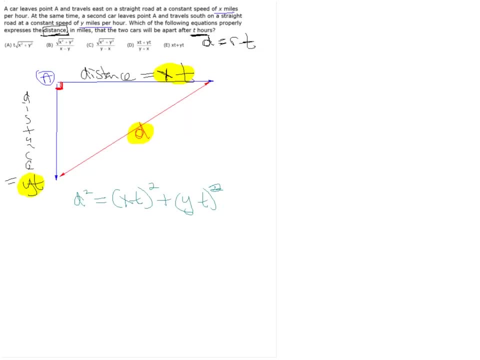 okay, so now we're just down to some. okay, so now we're just down to some exponent rules, right? so remember that. exponent rules, right. so remember that exponent rules, right. so remember that those twos belong to all of the. those twos belong to all of the. 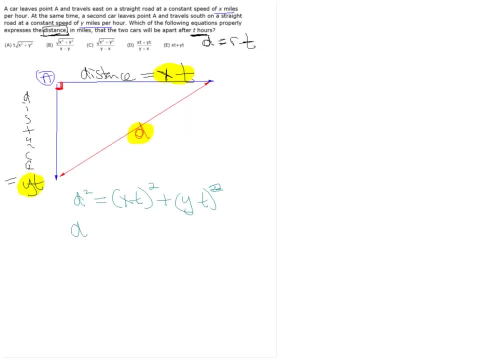 those twos belong to all of the characters inside, characters inside, characters inside. so we would say so. we would say so. we would say: the distance squared is equal to x. the distance squared is equal to x. the distance squared is equal to x squared squared. squared multiplied by t squared. 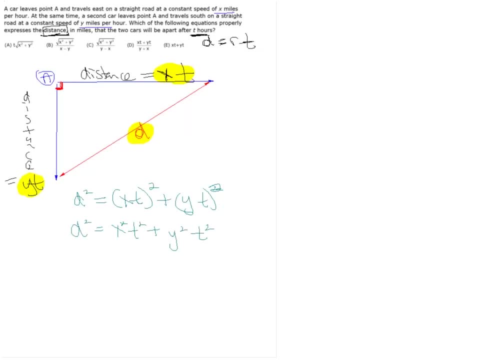 multiplied by t squared, multiplied by t squared plus y squared, multiplied by t squared plus y squared, multiplied by t squared plus y squared multiplied by t squared. okay, okay, okay, um again. take every factorable um again. take every factorable um again. take every factorable opportunity you can. 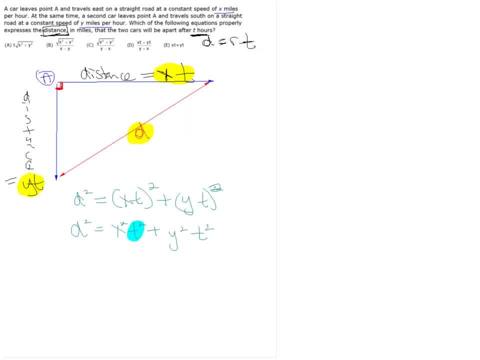 opportunity you can, opportunity you can. you can see here that in these two terms. you can see here that in these two terms. you can see here that in these two terms, they both share the t squared variable. they both share the t squared variable. they both share the t squared variable so immediately, without really giving it. 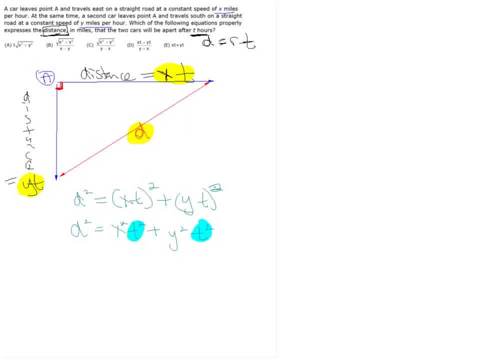 so immediately, without really giving it so immediately, without really giving it any thought we're going to pluck that, any thought we're going to pluck that, any thought we're going to pluck that right out of there. pull that right now, right out of there, pull that right now. 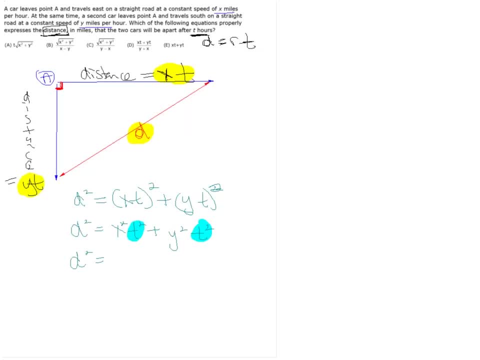 right out of there, pull that right now. so we'll say d squared. so we'll say d squared. so we'll say d squared is equal to t squared, and then inside of is equal to t squared, and then inside of is equal to t squared, and then inside of there we have x squared plus. 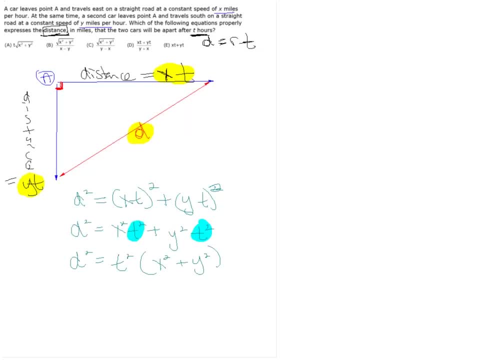 there we have x squared plus. there we have x squared plus y squared, y squared, y squared, and of course we're solving for d. so and of course we're solving for d so and of course we're solving for d. so we're going to take the square root of. 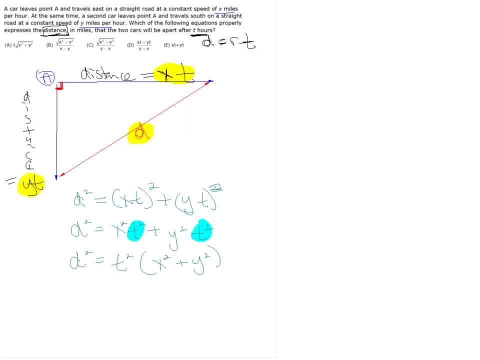 we're going to take the square root of, we're going to take the square root of both sides, both sides, both sides. so when we do that, so when we do that, so when we do that, we have d is equal to t. we have d is equal to t. 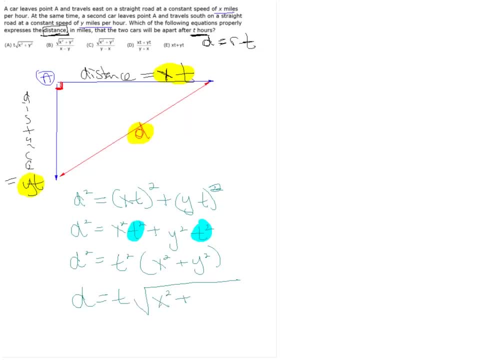 we have: d is equal to t times the square root of x squared times the square root of x squared times the square root of x squared plus y squared. now, before we summarize the problem now, before we summarize the problem now, before we summarize the problem, students always say well, 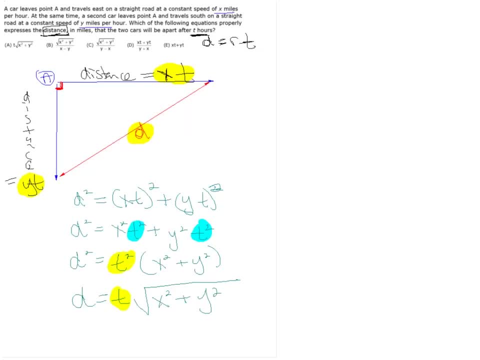 students always say well. students always say well. why did the t squared become p? why did the t squared become p? why did the t squared become p? but the rest of this became just what. but the rest of this became just what. but the rest of this became just what it was before, but under the radical. 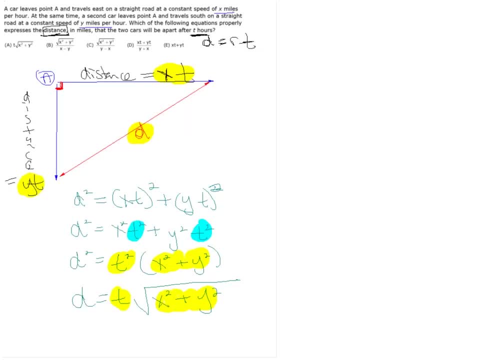 it was before, but under the radical. it was before, but under the radical, and the answer is that. and the answer is that, and the answer is that i'll kind of do it over here to the. i'll kind of do it over here to the. i'll kind of do it over here to the side of pink. well, 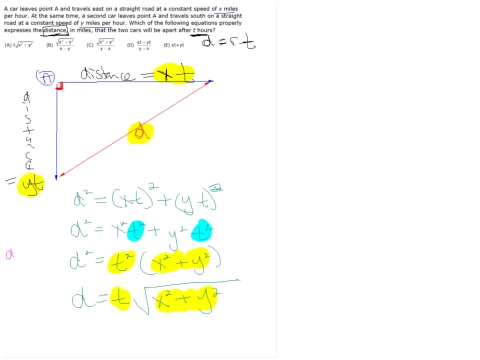 side of pink, well, side of pink, well. if you think about it, what you did is you. if you think about it, what you did is you. if you think about it, what you did is you. took the square root, took the square root, took the square root of the entire. 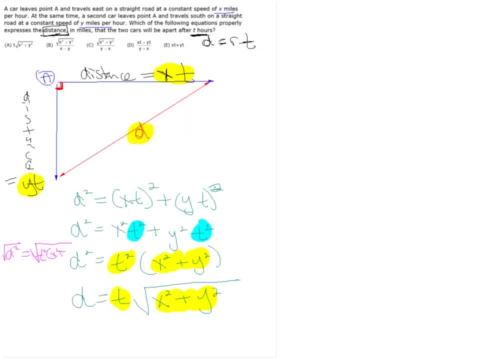 of the entire, of the entire. took the square root of the entire, took the square root of the entire, took the square root of the entire. equation, equation, equation. and the square root of t squared is, and the square root of t squared is, and the square root of t squared is just t, and the square root of d squared. 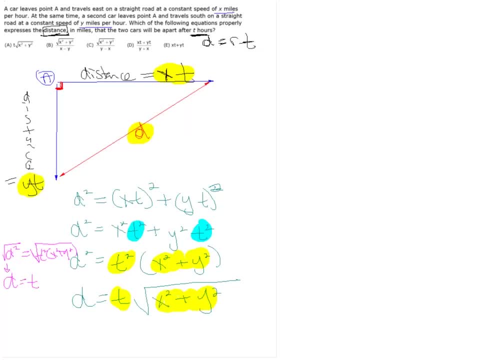 just t. and the square root of d squared, just t. and the square root of d squared is just d right. so is just d right, so is just d right. so square root of d squared is d square root. square root of d squared is d square root. 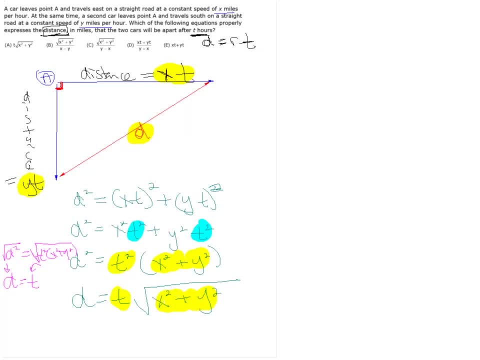 square root of d squared is d. square root of t squared is p of t squared is p of t squared is p. however, this, the x plus y squared had to. however, this, the x plus y squared had to. however, this, the x plus y squared had to stay under the radical. 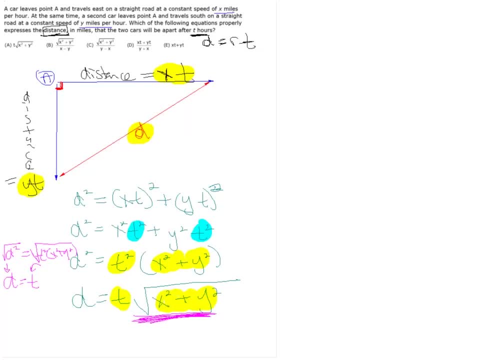 stay under the radical. stay under the radical because remember the order of operation, because remember the order of operation, because remember the order of operation dictates that, dictates that dictates that we must resolve any calculations, we must resolve any calculations, we must resolve any calculations under the radical, under the radical. 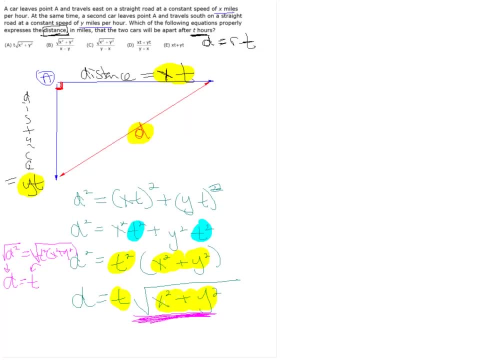 we must resolve any calculations under the radical before we actually take the radical, before we actually take the radical, before we actually take the radical, okay. so obviously you know for some of okay, so obviously you know for some of okay, so obviously you know for some of you, that may be a discussion for another. 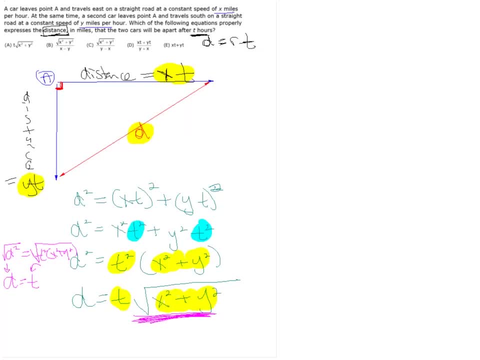 you- that may be a discussion for another you- that may be a discussion for another day, day, day, but at least take note of that and be on. but at least take note of that and be on. but at least take note of that and be on the lookout for that. 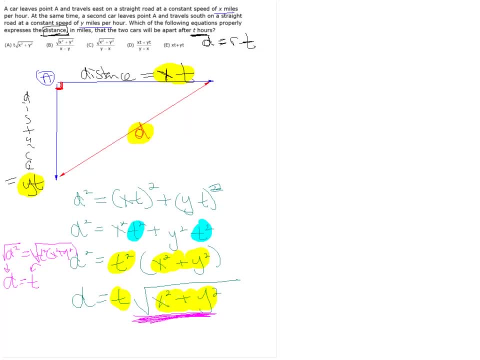 the lookout for that. the lookout for that. let's see, do we have that answer choice? let's see, do we have that answer choice? let's see, do we have that answer choice up there? let's scroll up up there. let's scroll up up there. let's scroll up. yeah, we do that's answer choice a. 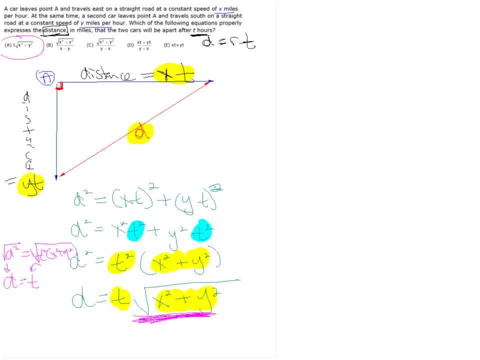 yeah, we do that's answer choice a. yeah, we do that's answer choice a. okay, so again in this problem. okay, so again in this problem, okay, so again in this problem. all we did was we carefully decoded the all we did was we carefully decoded the all we did was we carefully decoded the word problem. 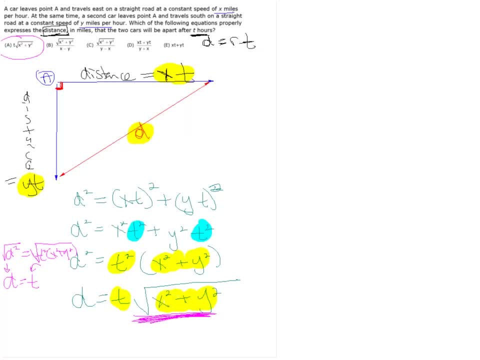 word problem, word problem, and we integrated in the distance and we integrated in the distance and we integrated in the distance formula, formula, formula, um and, as i said, it's, it's important um and, as i said, it's, it's important um and, as i said, it's it's important when you work in geometry questions to 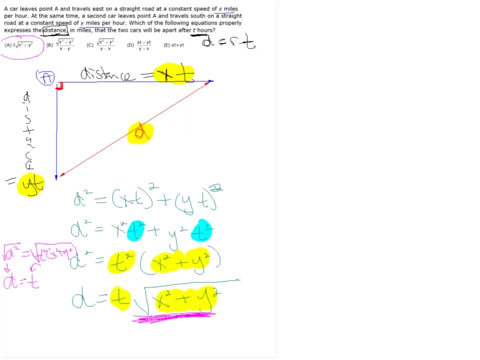 when you work in geometry questions to: when you work in geometry questions: to not be shocked if you have other topics. not be shocked if you have other topics. not be shocked if you have other topics or concepts that get okay, why don't you catch up with that? 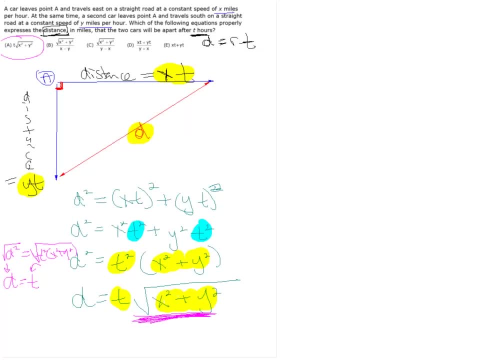 okay, why don't you catch up with that? okay, why don't you catch up with that? take any notes you want to take down on. take any notes you want to take down on. take any notes you want to take down on that guy. okay, let's do this guy. 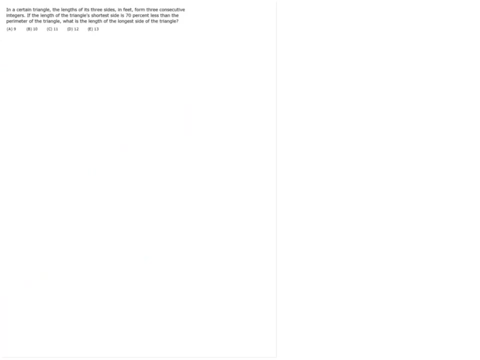 okay, let's do this guy. okay, let's do this guy not that difficult, so i'm going to shoot. not that difficult, so i'm going to shoot. not that difficult, so i'm going to shoot for a strict two minutes on this guy, for a strict two minutes on this guy. 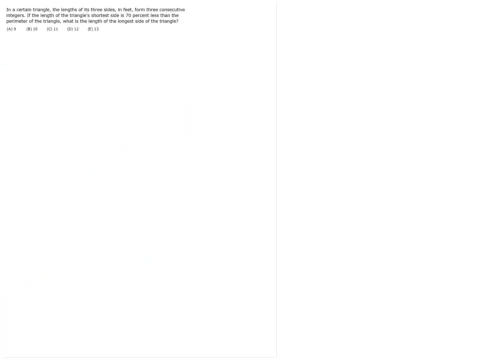 for a strict two minutes on this guy starting, starting, starting. okay guys, uh, that was about two minutes. okay guys, uh, that was about two minutes. okay guys, uh, that was about two minutes. and uh, yeah, definitely fill out the. and. uh, yeah, definitely fill out the. and uh, yeah, definitely fill out the feedback form. as i always say, we'll um. 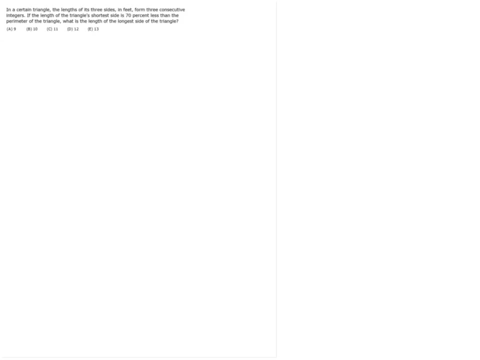 feedback form. as i always say, we'll um feedback form. as i always say, we'll um try and tailor these webinars. to try and tailor these webinars. to try and tailor these webinars to whatever interests or deficiencies, whatever interests or deficiencies, whatever interests or deficiencies people have. 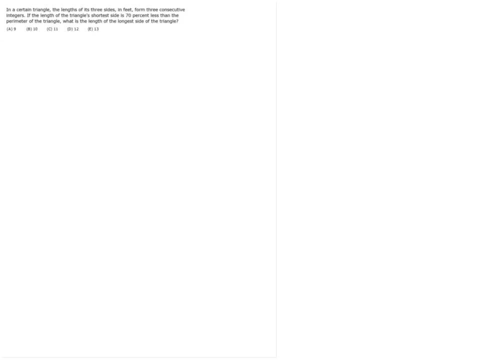 people have people have anyone really knows you fill out that. anyone really knows you fill out that. anyone really knows you fill out that form. so please make sure you do that form. so please make sure you do that form. so please make sure you do that. after the webinar: 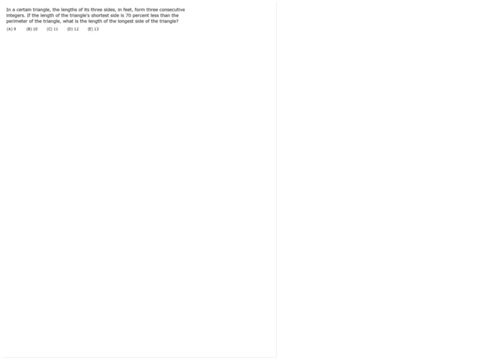 after the webinar. after the webinar: so for this problem. so we have a so for this problem. so we have a so for this problem. so we have a certain triangle and the lengths of the certain triangle and the lengths of the certain triangle and the lengths of the three sides form consecutive integers. 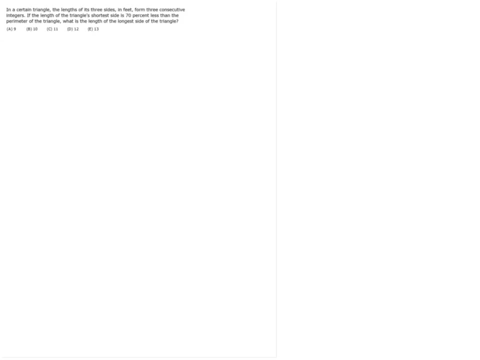 three sides form consecutive integers. three sides form consecutive integers: um. let's stop right there. um. let's stop right there. um. let's stop right there. so it's important to be able to: so it's important to be able to, so it's important to be able to algebraically express: algebraically express. algebraically express three consecutive integers, and by that three consecutive integers, and by that three consecutive integers, and by that they mean like, they mean like. they mean like one, two, three, one, two, three, one, two, three or five, six, seven, or or five, six, seven or. 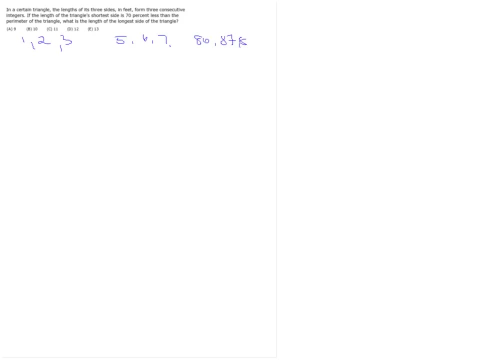 or five, six, seven or eighty six, eighty six, eighty six, seven, eighty eight, seven, eighty eight, seven, eighty, eight, um, anything where you have um, anything where you have um, anything where you have three numbers that are consecutive, three numbers that are consecutive, three numbers that are consecutive. okay, 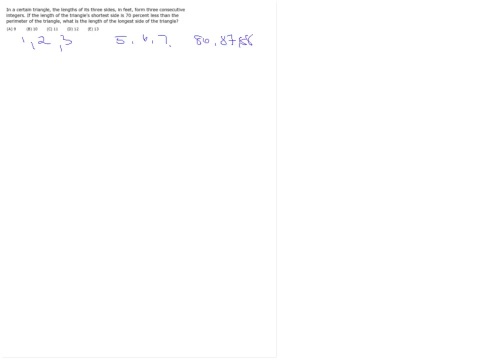 okay, okay. so the way to write this algebraically, so the way to write this algebraically, so the way to write this algebraically- and this is important- is to say the, and this is important- is to say the, and this is important is to say the numbers are n. 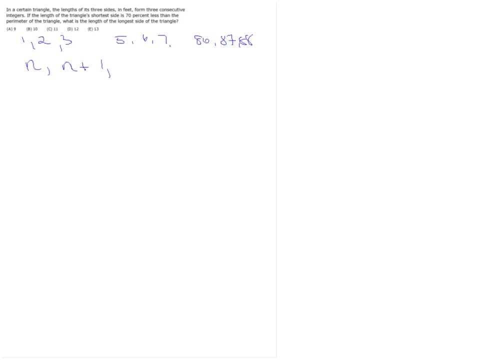 numbers are n, numbers are n. you could say: the next number is n plus. you could say: the next number is n plus. you could say: the next number is n plus one, one one, and then the next number is n plus two, and then the next number is n plus two. 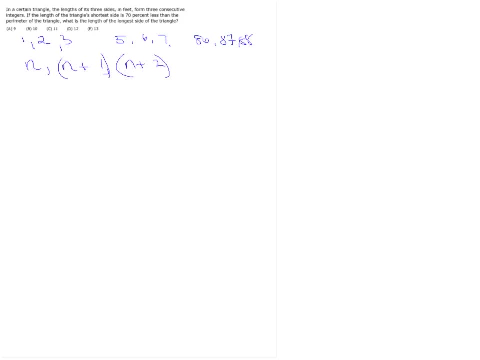 and then the next number is n plus two. that's how we would algebraically say. that's how we would algebraically say: that's how we would algebraically say: three consecutive. you could use x you. three consecutive. you could use x you three consecutive. you could use x you three consecutive integers. 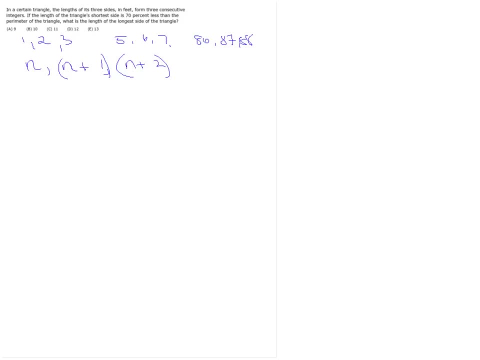 three consecutive integers, three consecutive integers. okay, so this triangle, it says the length. okay, so this triangle, it says the length. okay, so this triangle, it says the length of its three sides, of its three sides, of its three sides, form three consecutive integers, form three consecutive integers, form three consecutive integers. it says, if the length of the triangle's 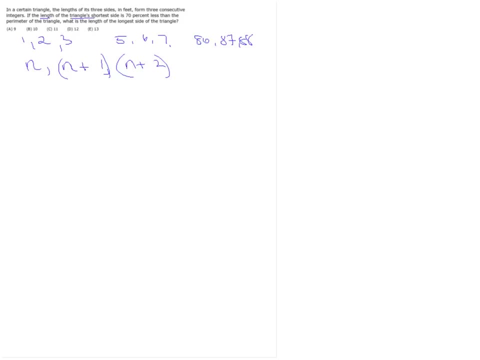 it says: if the length of the triangle's. it says: if the length of the triangle's shortest side is 70, shortest side is 70, shortest side is 70, less than the perimeter of the triangle, less than the perimeter of the triangle, less than the perimeter of the triangle, what is the length of the longest side? 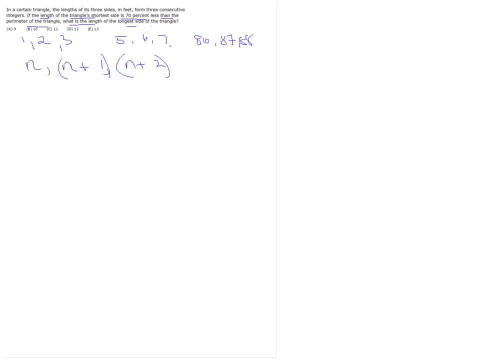 what is the length of the longest side? what is the length of the longest side? so if you think about it, so this, so if you think about it so this, so if you think about it, so this triangle will, triangle, will triangle will definitely not, definitely not, definitely not be a scale, but if we have 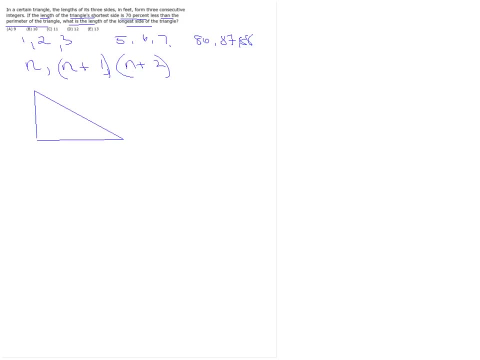 be a scale. but if we have, be a scale. but if we have the triangle that we're dealing with, the triangle that we're dealing with, the triangle that we're dealing with especially, we could say the sides are especially. we could say the sides are especially, we could say the sides are, you know, n. 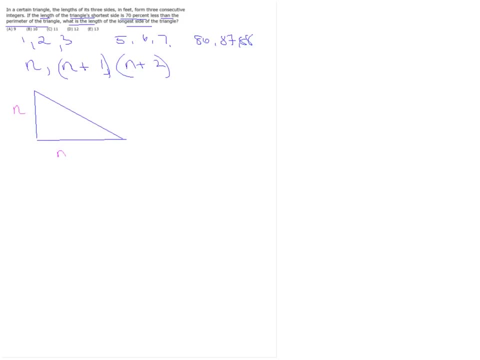 you know n, you know n. we could say the next longer side was n. we could say the next longer side was n. we could say the next longer side was n plus one plus one plus one, and the next the longest side would be n and the next the longest side would be n. 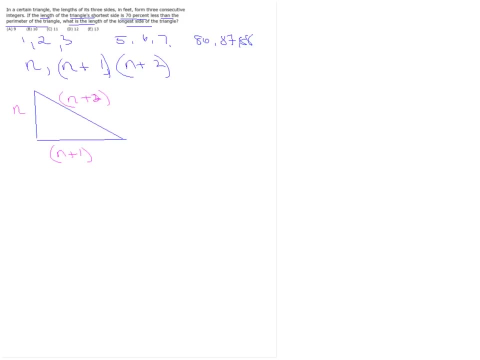 and the next, the longest side would be n plus two. so just remember: in a triangle plus two, so just remember. in a triangle plus two, so just remember. in a triangle, hypotenuse has to be the longest side. hypotenuse has to be the longest side. 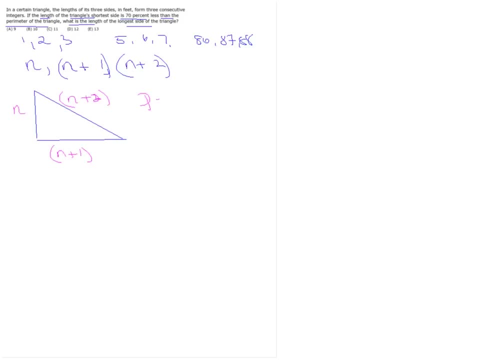 hypotenuse has to be the longest side, then what that means is the perimeter, then what that means is the perimeter. then what that means is the perimeter is simply n, is simply n, is simply n plus n plus one plus n plus one plus n plus one plus n plus two. 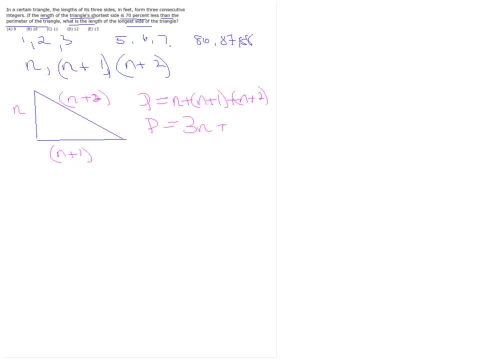 plus n plus two, plus n plus two, so then the perimeter is three and plus. so then the perimeter is three and plus. so then the perimeter is three and plus three, three, three. okay, algebraically the perimeter can. okay, algebraically, the perimeter can. okay. algebraically, the perimeter can be represented by three and plus three. 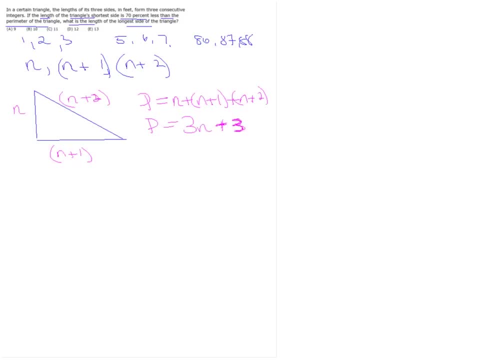 be represented by three and plus three, be represented by three and plus three. so what it says is the shortest side is so what it says is the shortest side is so what it says is the shortest side is 70 percent, 70 percent, 70 percent less than the perimeter. 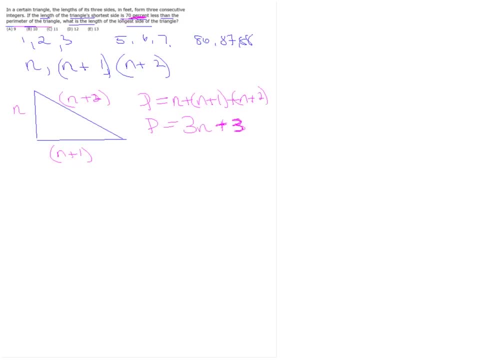 less than the perimeter. less than the perimeter. so any time we know that something is so, any time we know that something is so, any time we know that something is 70 percent, 70 percent, 70 percent, less, it's really helpful to say to less, it's really helpful to say to. 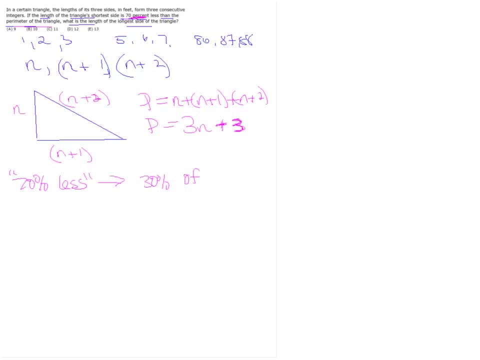 less. it's really helpful to say to ourselves: well, that means ourselves, well, that means ourselves. well, that means 30 percent, oh right, 30 percent. oh right, 30 percent, oh right. so if you're, if you're 70 percent less, so if you're, if you're 70 percent less. 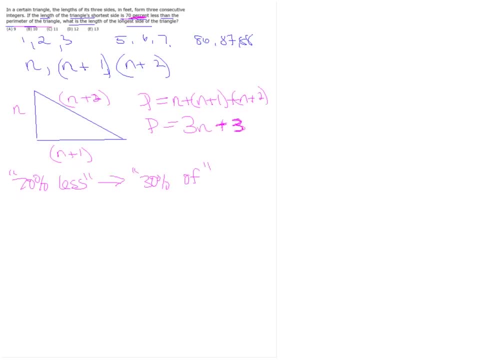 so if you're, if you're 70 percent less, you're 30 percent of, you're 30 percent of, you're 30 percent of right, say you don't save a hundred right, say you don't save a hundred right, say you don't save a hundred dollars if you're. 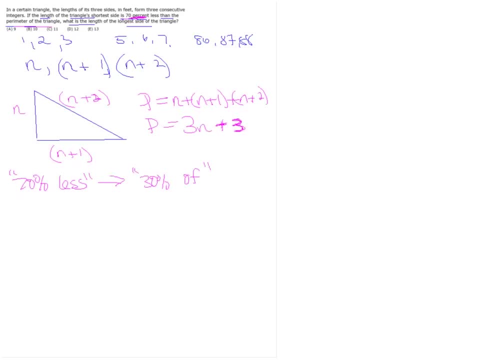 dollars. if you're dollars. if you're, lose 70 of that. you have 30. lose 70 of that. you have 30, lose 70 of that. you have 30 percent left, percent left, percent left. okay, so we're going to decode this watch. okay, so we're going to decode this watch. 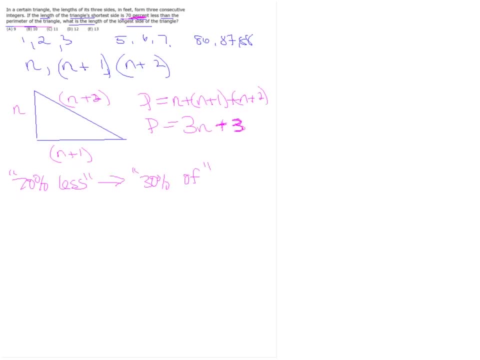 okay, so we're going to decode this watch as we write the equation, as we write the equation, as we write the equation. so we are going to say that the triangle, so we are going to say that the triangle. so we are going to say that the triangle, shortest side, which remember by. 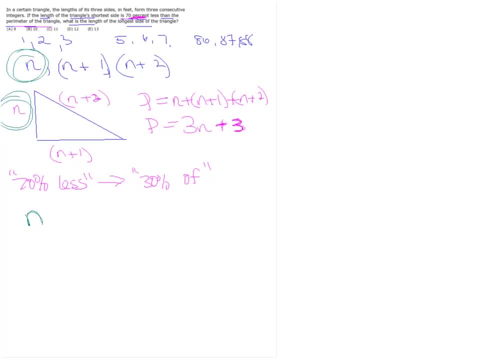 shortest side which remember by shortest side, which remember by definition, definition, definition n, n, n. and the definition by definition, we let. and the definition by definition, we let. and the definition by definition, we let. the shortest side be n, the shortest side be n, the shortest side be n. so the triangle shortest side is: 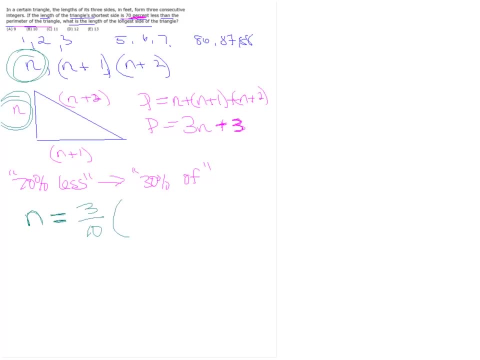 so the triangle shortest side is. so the triangle shortest side is equals, equals, equals: 30 percent, 30 percent, 30 percent of of the perimeter of the triangle, the perimeter of the triangle, the perimeter of the triangle. at this point, you just have a very basic. at this point, you just have a very basic. 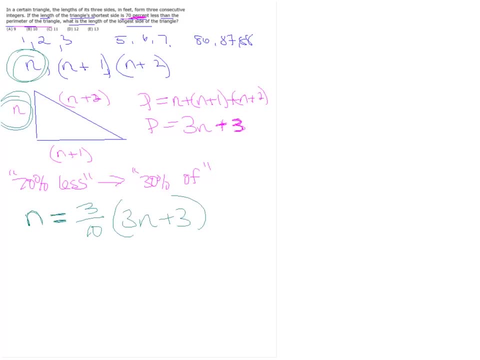 at this point you just have a very basic linear equation. linear equation, linear equation, we can, we can, we can. our goal would be to. our goal would be to. our goal would be to eliminate the fraction quickly. eliminate the fraction quickly, eliminate the fraction quickly, or you can multiply the. 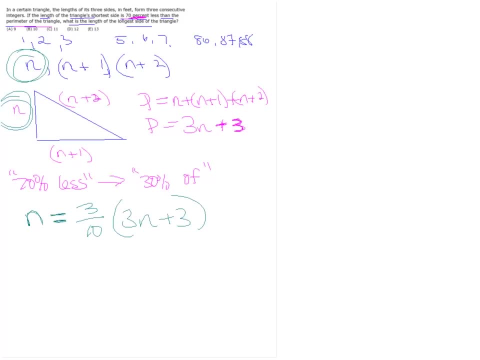 or you can multiply the, or you can multiply the three-tenth through, three-tenth through, three-tenth through. it's up to you. it depends on what you'd. it's up to you. it depends on what you'd. it's up to you. it depends on what you'd like to do so. 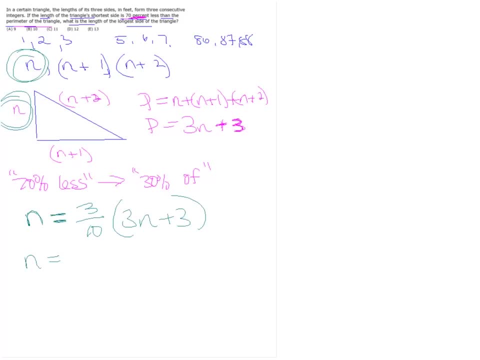 like to do so, like to do so. let's put it through. so, let's put it through, so, let's put it through. so let's say: this becomes nine tenths. so let's say: this becomes nine tenths. so let's say: this becomes nine tenths. so point nine n. 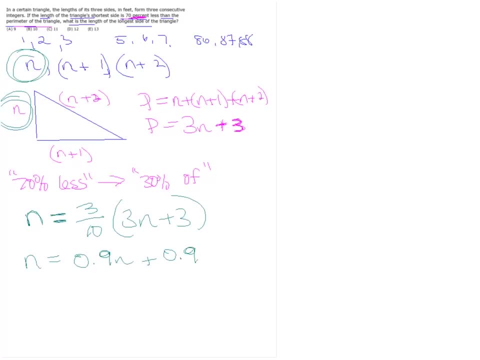 point nine, n point nine, n plus plus plus zero point nine right nine tenths zero point nine right nine tenths zero point nine right nine tenths um. we can then um. we can then um. we can then bring the, bring the, bring the. let's see what the next is. 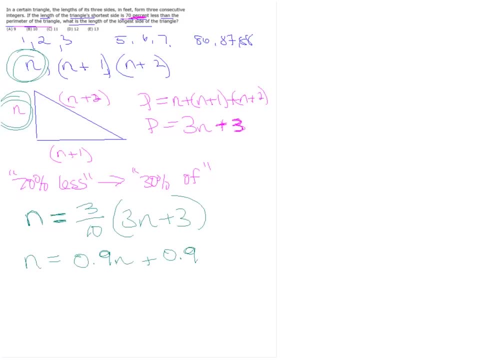 let's see what the next is. let's see what the next is. let's bring the two terms with the n. let's bring the two terms with the n. let's bring the two terms with the n together, so we'll say n. together, so we'll say n. 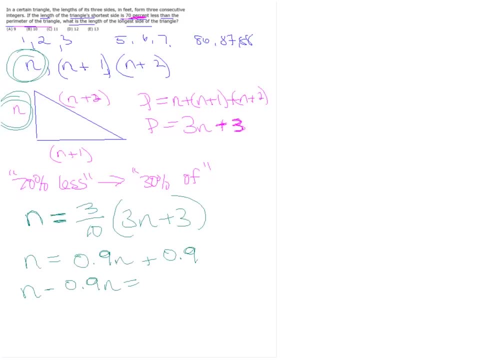 together. so we'll say n minus minus minus zero point nine n zero point nine n zero point nine. n is equal to 0.9, is equal to 0.9, is equal to 0.9. okay, so the reason why i did that is: 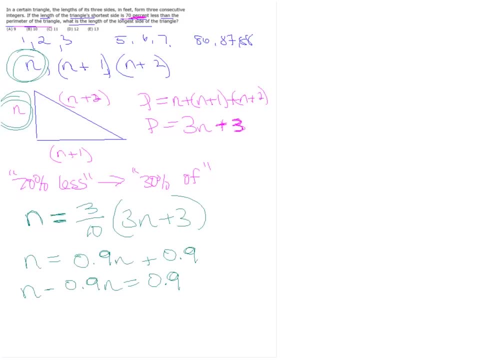 okay. so the reason why i did that is okay. so the reason why i did that is because obviously we're going to solve, because obviously we're going to solve, because obviously we're going to solve n here, and so n minus nine tenths of n n here, and so n minus nine tenths of n. 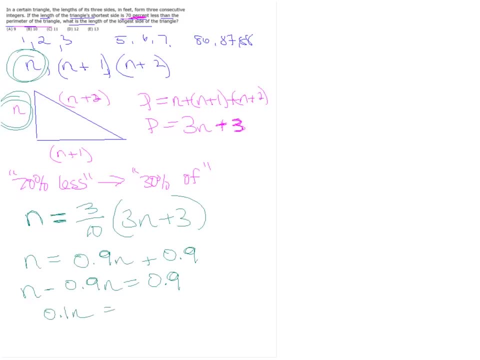 n here, and so n minus nine tenths of n is one. tenth of n is one. tenth of n is one. tenth of n is equal to 0.9, is equal to 0.9, is equal to 0.9, so n here is equal. 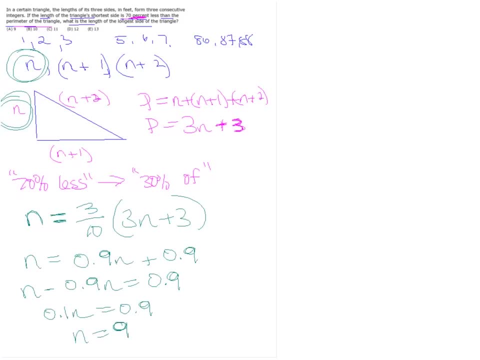 so n here is equal. so n here is equal to 9. to 9. to 9.. and you didn't have to solve it the way i and you didn't have to solve it the way i and you didn't have to solve it the way i did. most of the time i actually don't. 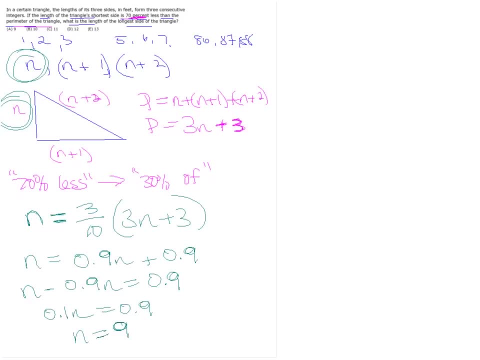 did most of the time. i actually don't did most of the time. i actually don't use decimals just a moment. i like use decimals just a moment. i like use decimals just a moment. i like writing the decimals out, writing the decimals out, writing the decimals out, these fractions, because there's been a lot. 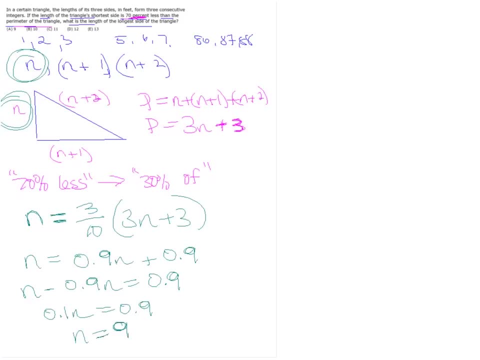 these fractions, because there's been a lot these fractions, because there's been a lot of different techniques. whatever makes of different techniques, whatever makes of different techniques, whatever makes sense for you, but we see n is equal to sense for you, but we see n is equal to. 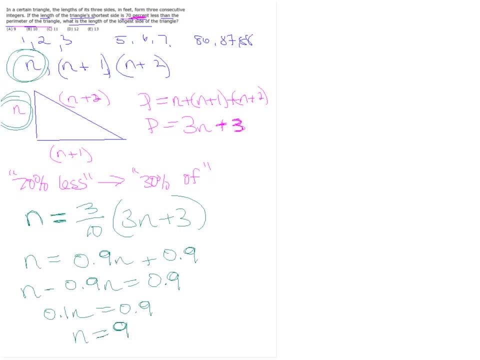 sense for you. but we see, n is equal to nine and nine and nine and, as jeff told you earlier, like if you're as jeff told you earlier, like if you're as jeff told you earlier, like if you're in a rush, you can bet your answer a. 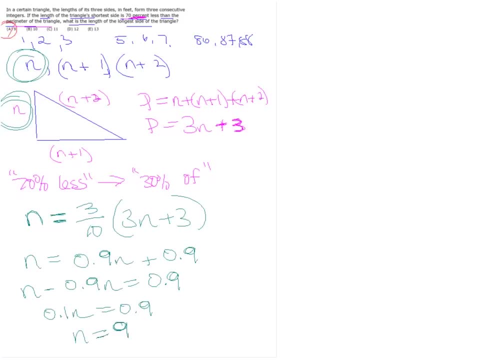 in a rush, you can bet your answer: a. in a rush, you can bet your answer a: um, but a is not the answer. so on the um, but a is not the answer. so on the um, but a is not the answer. so on the test. a lot of trap answers are our. 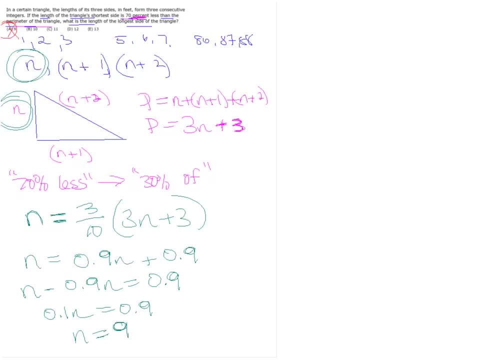 test. a lot of trap answers are our test. a lot of trap answers are our strategic values. meaning you know they're strategic values. meaning you know they're strategic values. meaning you know they're not like values that are not like values that are not like values that are insignificant in the problem, but they're. insignificant in the problem. but they're insignificant in the problem, but they're like, okay, i just did a lot of steps and i like, okay, i just did a lot of steps and i like, okay, i just did a lot of steps and i got this answer. got this answer. 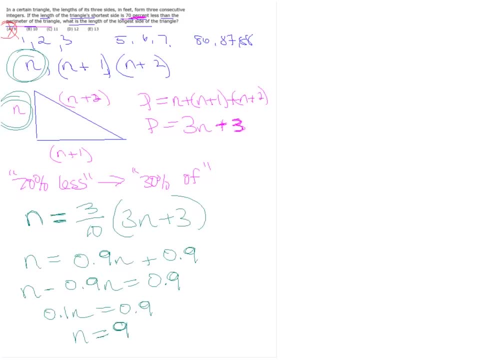 got this answer and you see the answer up there. well, you and you see the answer up there. well, you and you see the answer up there. well, you got to make sure that the answer you're got, to make sure that the answer you're got, to make sure that the answer you're picking is actually what's being asked. 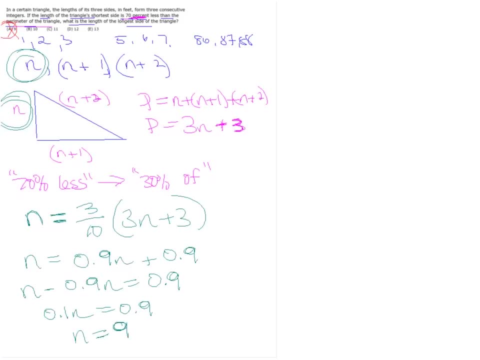 picking is actually what's being asked. picking is actually what's being asked, okay, so you have the value of n, which okay. so you have the value of n, which okay. so you have the value of n, which is the is the is the length of the shortest side, but obviously 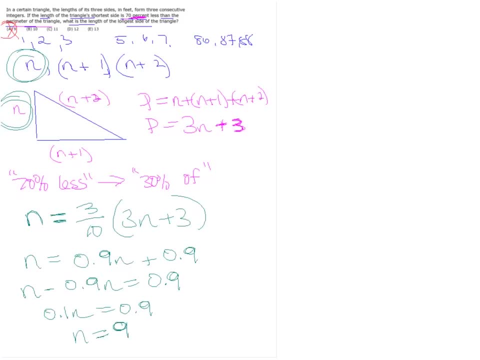 length of the shortest side, but obviously length of the shortest side. but obviously the question asks, the question asks. the question asks: what's the length of the longest side? what's the length of the longest side? what's the length of the longest side? and the longest side was expressed as: 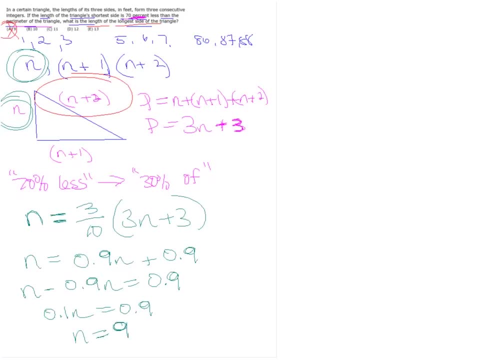 and the longest side was expressed as: and the longest side was expressed as 10 plus 2, so that makes the longest size 10 plus 2. so that makes the longest size 10 plus 2. so that makes the longest size actually 11.. 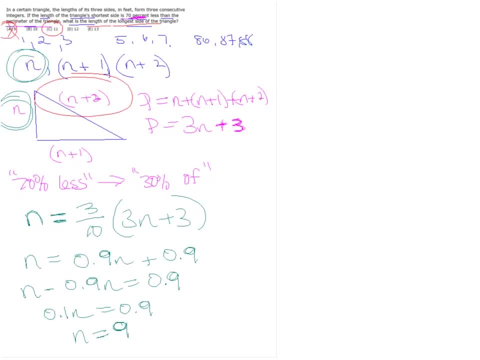 actually 11.. actually 11.. now i would guess i would say five. now i would guess i would say five. now i would guess i would say five to 10 of wrong answers and students. i to 10 of wrong answers and students. i to 10 of wrong answers and students. i have results from doing something like: 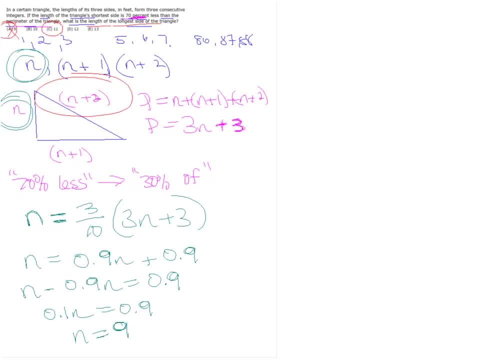 have results from doing something like. have results from doing something like that, that, that, right. so actually getting n equals nine, right. so actually getting n equals nine, right. so actually getting n equals nine. and picking nine is the answer, not you. and picking nine is the answer, not you. 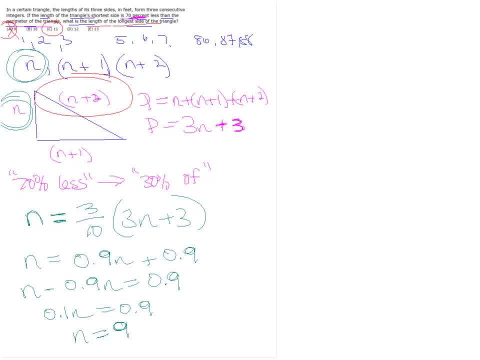 and picking nine is the answer? not, you know, kind of forgetting that, what's know, kind of forgetting that what's know, kind of forgetting that what's really being asked is what's the longest really being asked is what's the longest really being asked is what's the longest side. 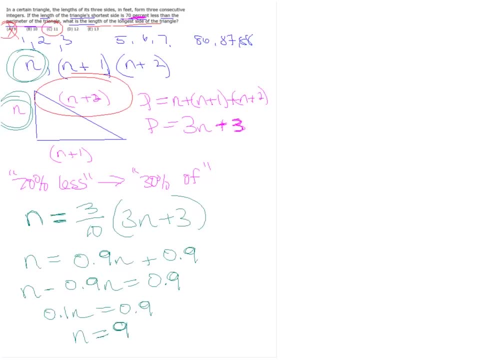 side side. so obviously you don't want to do all. so obviously you don't want to do all. so obviously you don't want to do all that work and then be penalized because that work and then be penalized because that work and then be penalized because you didn't carefully. 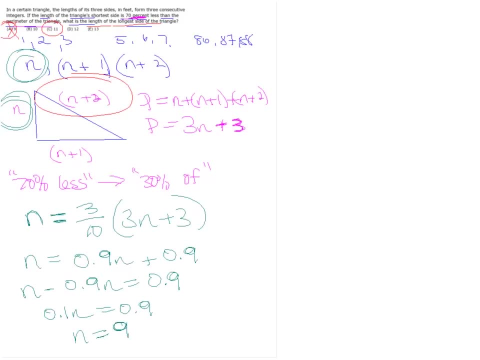 you didn't carefully. you didn't carefully answer what the questions. actually, okay, so that's all for me, jeff, i'm gonna okay. so that's all for me, jeff, i'm gonna okay. so that's all for me, jeff, i'm gonna turn it back over to you with any last. 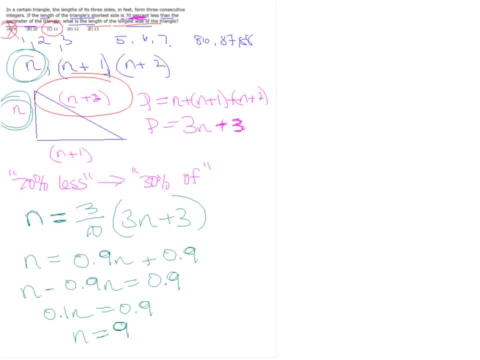 turn it back over to you with any last, turn it back over to you with any last words of wisdom or anything else. you want words of wisdom, or anything else you want words of wisdom, or anything else you want to mention, to mention, to mention. uh, yeah, well, just thanks again for coming. 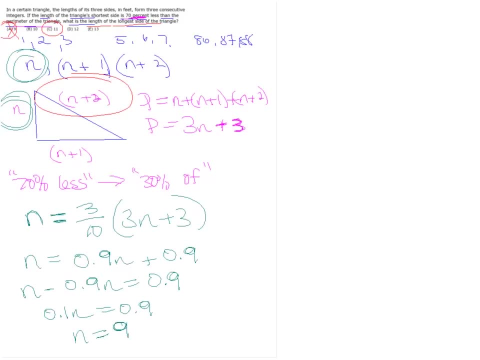 uh, yeah, well, just thanks again for coming. uh, yeah, well, just thanks again for coming, uh, this week. and uh like scott said, uh, uh, this week. and uh like scott said, uh, uh, this week. and uh like scott said, uh, definitely, fill out the feedback form um. 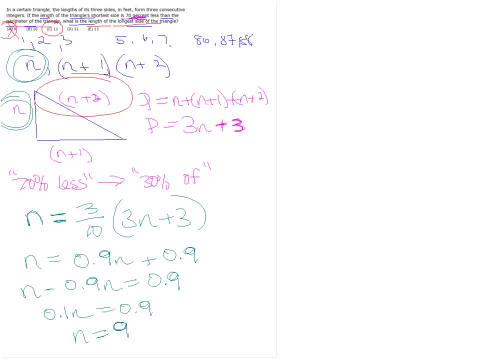 definitely fill out the feedback form. um. definitely fill out the feedback form. um. so we know you know your thoughts on, so we know you know your thoughts on, so we know you know your thoughts on these webinars and uh, as i said earlier, these webinars and uh, as i said earlier,